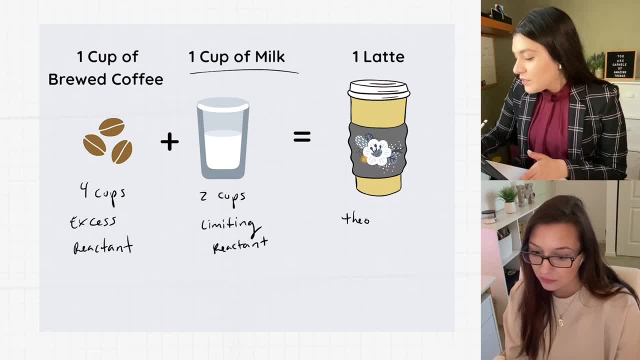 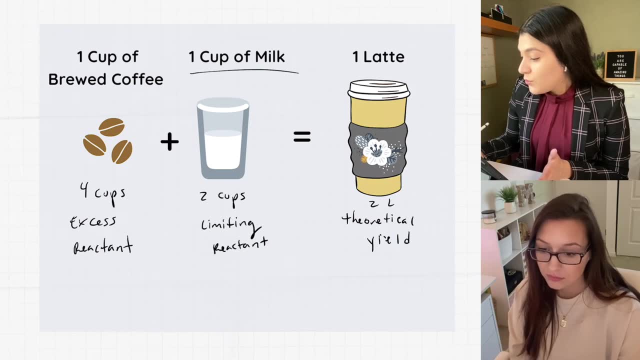 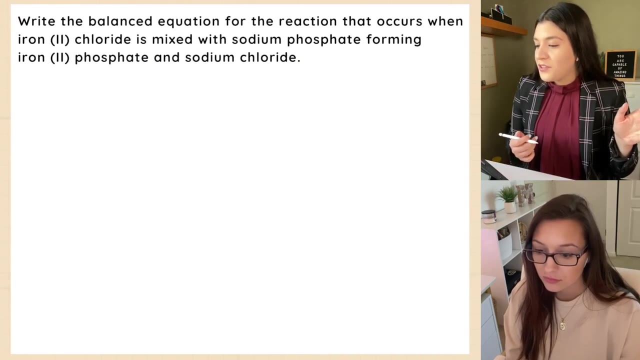 limiting reactant actually produces is then called Our theoretical yield. So in this case, our theoretical yield would have been, you know, two lattes that we could actually produce. Okay, Cool. So now that you understand the concept, let's put this into chemistry. Let's start off with just practicing. This is actually a good 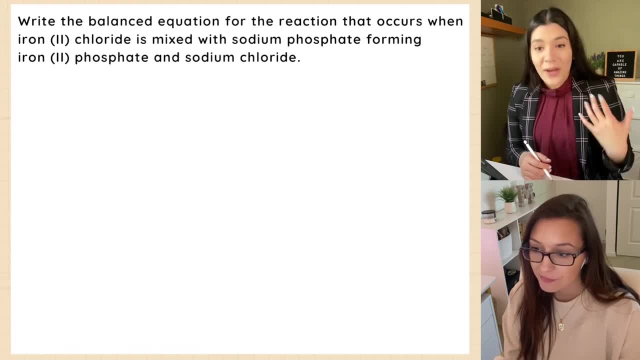 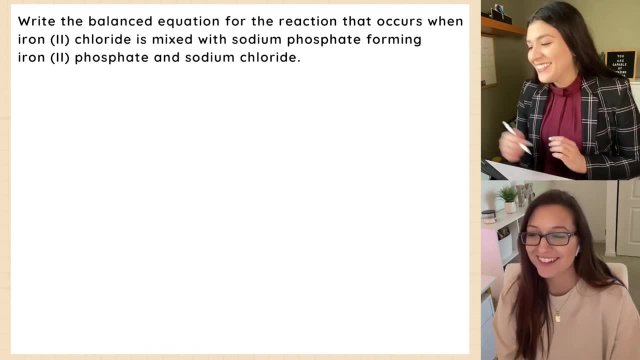 practice for us Practicing building equations, balancing them, and this is going back to naming. So, yeah, I thought we did away with that. We did not. We did not, And it's good practice for the final as well, All right. So this question. 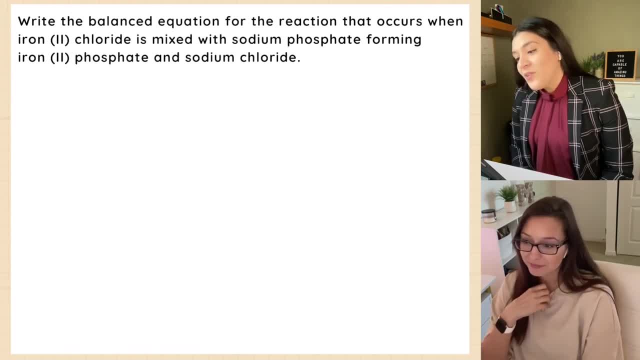 is asking us to write the balance equation for the reaction that occurs when iron 2 chloride is mixed with sodium phosphate, forming iron 2 phosphate and sodium chloride. So we need to go back to naming compounds. Let's just start off with how we would write the chemical formula for: 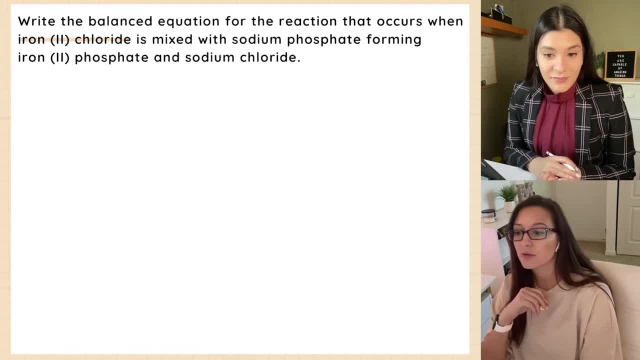 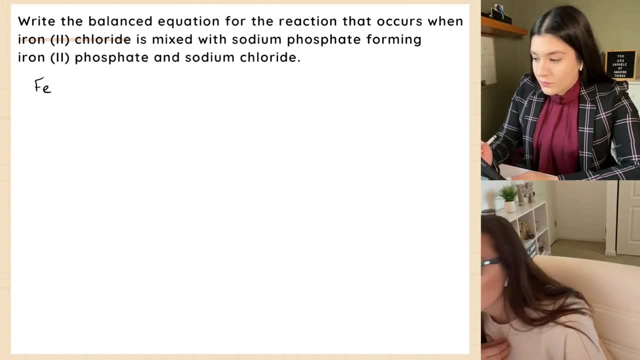 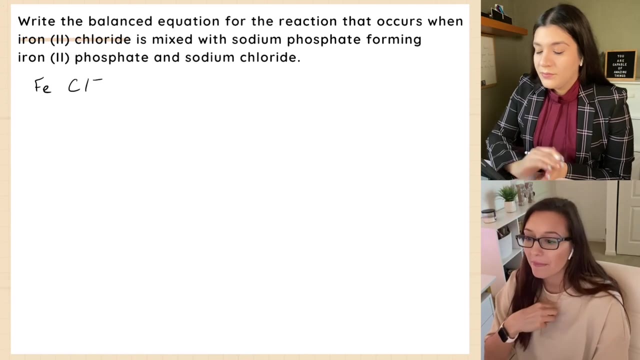 iron 2 chloride, Go for it. Okay, So we would write Fe for iron And then um and then Cl. Good, And then we try to take a negative 1 and a 2 plus What? Yeah, That's the Roman Numeril tells us the charges of the metal. 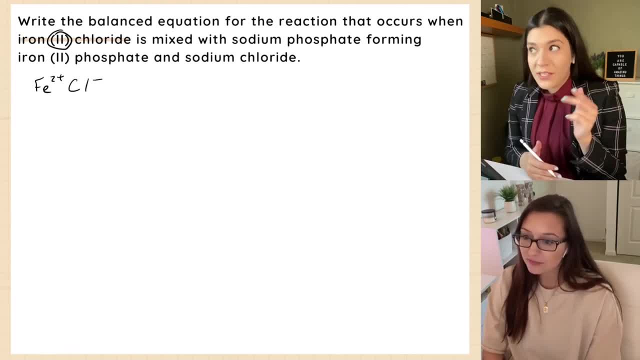 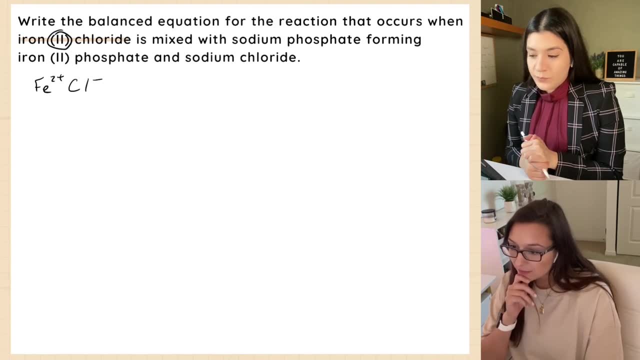 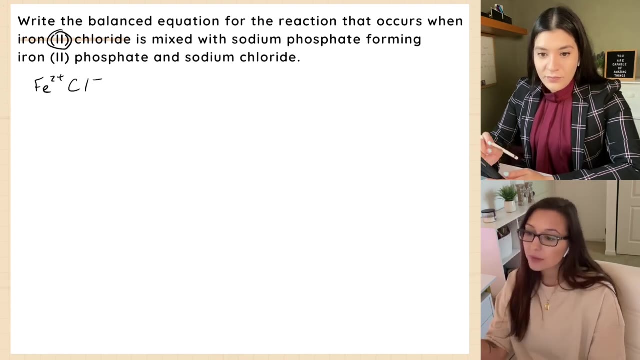 perfect. And then how? let's keep going. all right, balance out the charges and find a chemical formula. Okay, So we will. We're trying to explain this. I don't remember how you told me to do this. we're multiplying and then adding in the subscripts. 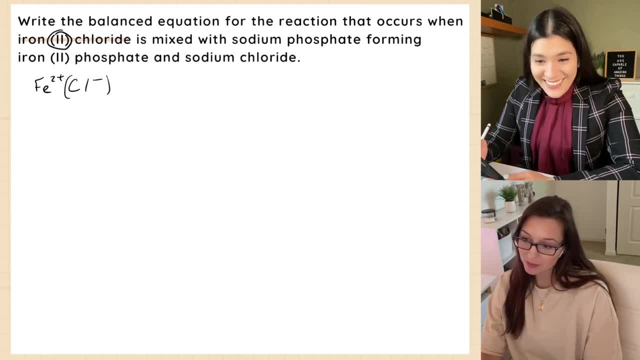 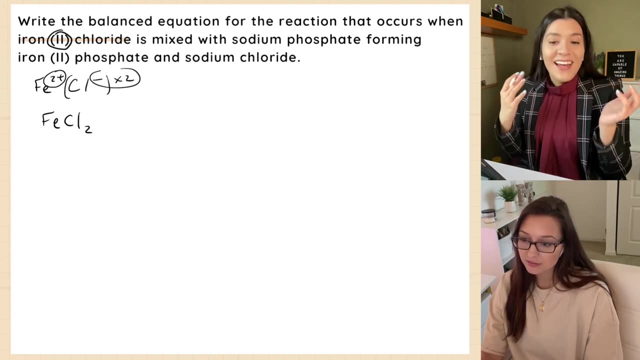 so correct. yeah, so we'll multiply that by two. good, because we want both of these numbers to be two. but essentially what what that means? right, when we're we had a subscript, that essentially kind of means that we're- excuse me, that essentially kind of means that we're multiplying two by that. 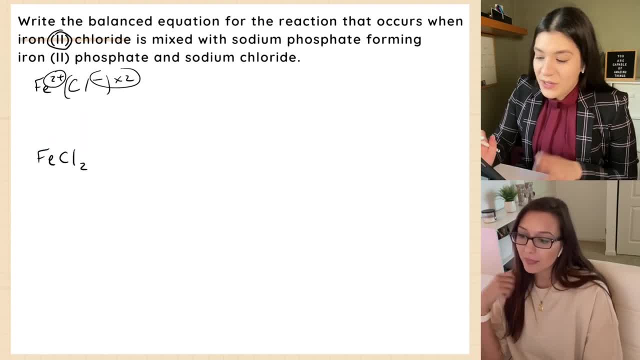 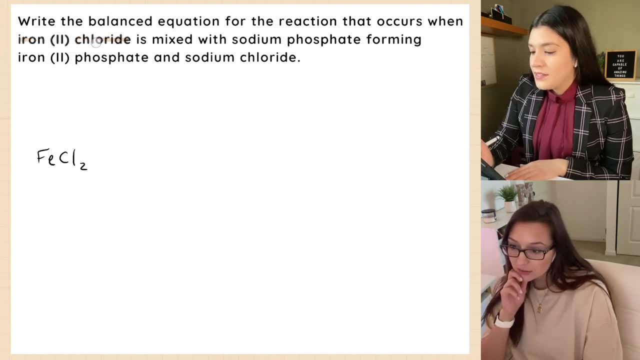 negative one charge, okay, cool. and then we never include the charges in the actual chemical formula. cool, okay, all right. and then next it's saying: iron two chloride is mixed. that tells us: okay, that's our second reactant is mixed with sodium phosphate, so sodium phosphate is our. 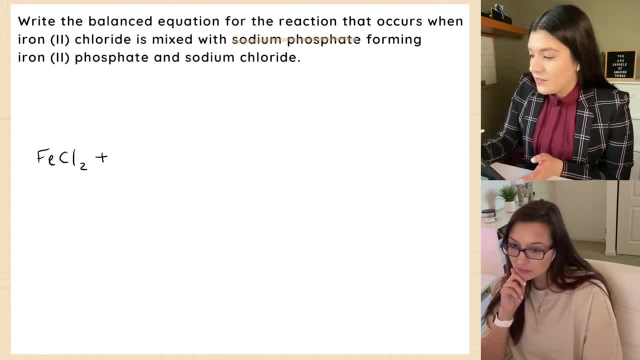 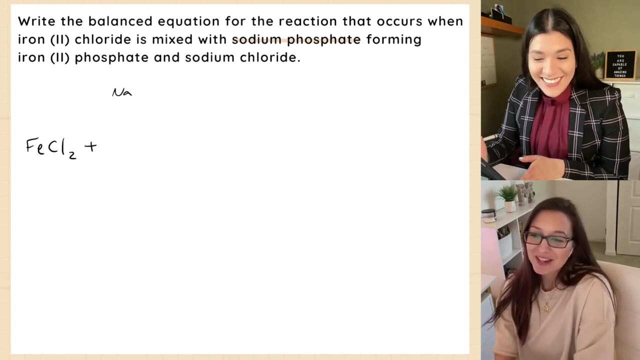 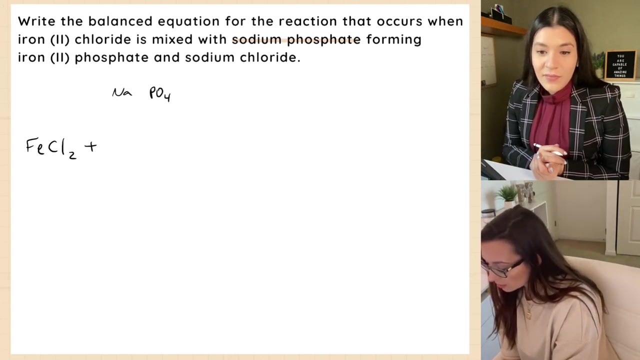 second reactant. and what is sodium phosphate? uh, okay, sodium phosphate. so we're gonna do n a mm-hmm sodium and phosphate is a polyatomic ion that we have to memorize, so po4, good, what's the charge of phosphate? um, oh no, it's not gonna. sadly, the periodic table won't save you there, so that. 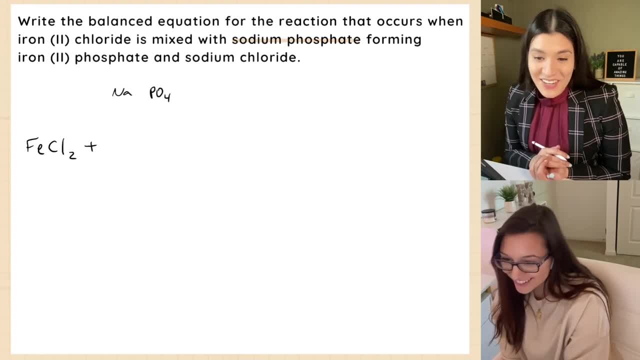 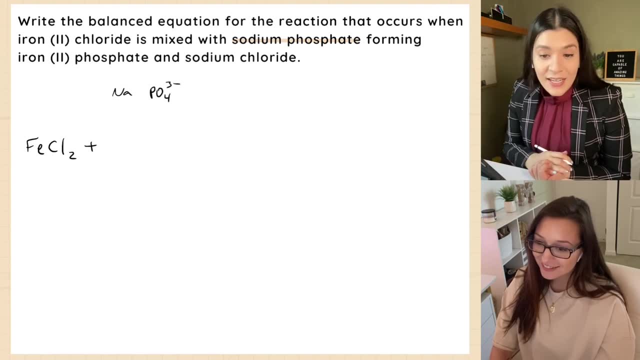 one is memory right: polyatomic ions and their charges. i know that one you just have to memorize. it's not going to be, it's not going to tell you know on the periodic table. so this is one that we had to know was a negative three, and then now with a. 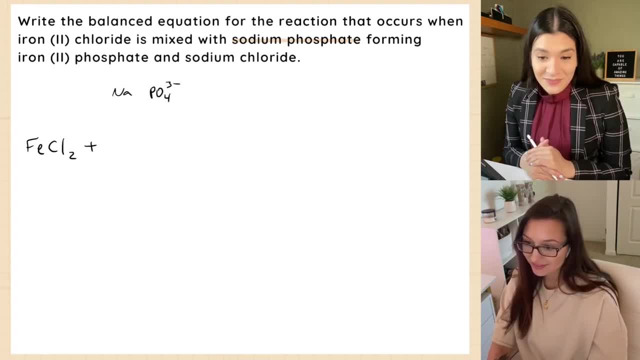 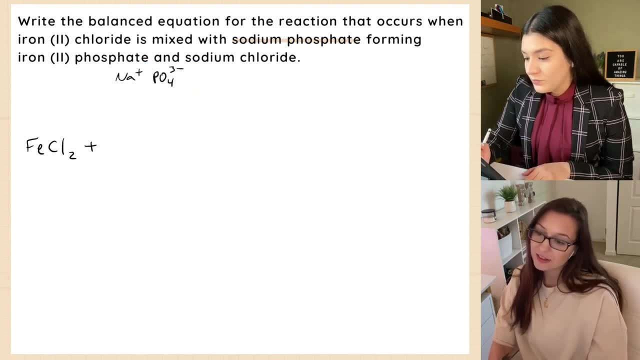 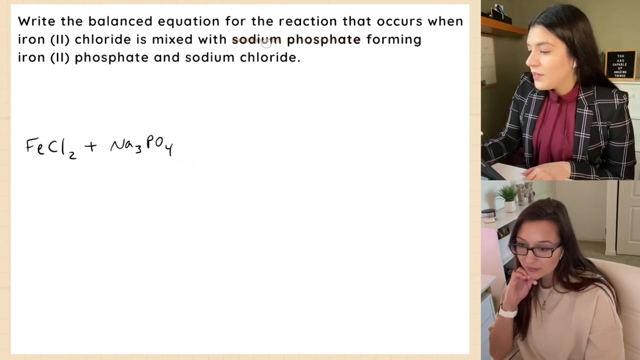 typical metal like sodium. yes, that one is on the periodic table. okay, so plus one. good, okay, keep going. how would i balance this? okay, so we have to multiply the sodium by three. so, um, we make it the subscript. so any three p, perfect, awesome. and then next i'm going to keep going and it's 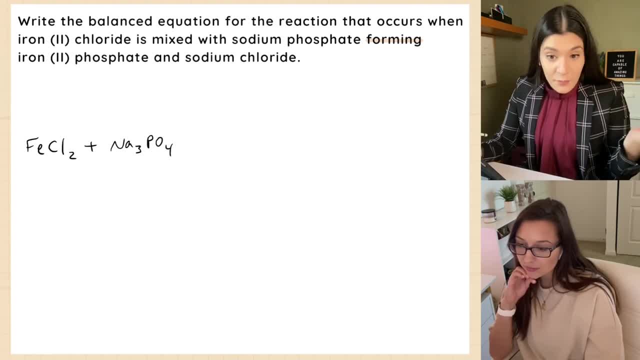 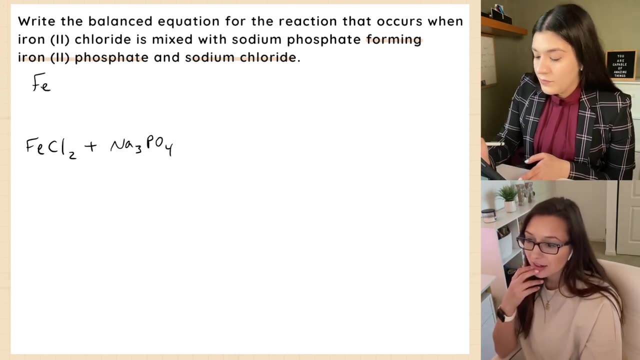 saying forming. so forming tells us: oh, the products are coming up, so this is our product. now our products are going to be iron two phosphate and sodium chloride. so let's start with iron two phosphate, okay. so, um, we do the iron, which is fe, and then the phosphate, the po4. 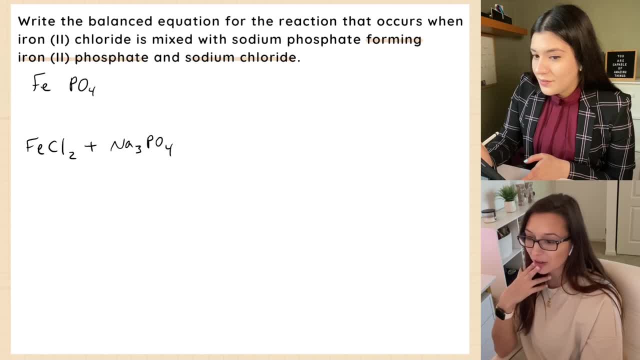 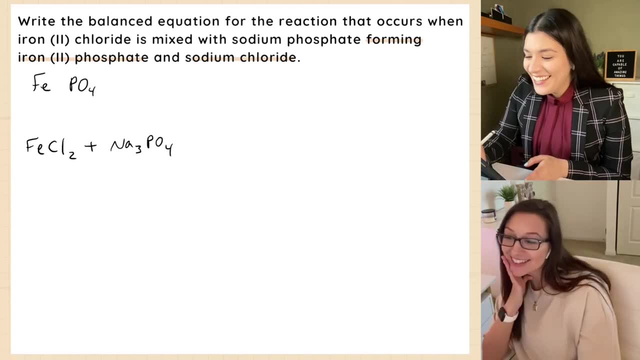 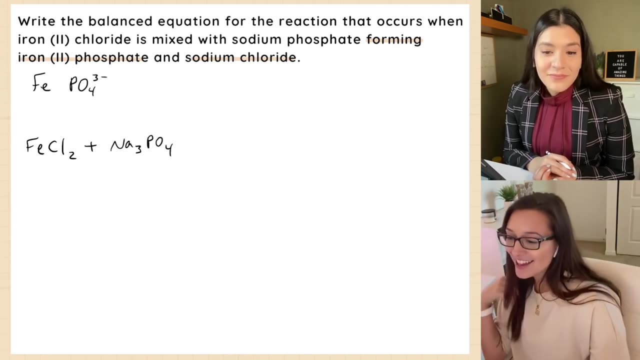 good with the charge that we know. now, yes, which was, i forgot that fast? three minus, oh yeah. okay, that's what i was gonna say, okay, um. and then the iron. we look at the charge of the periodic table. right, not necessarily, this has a roman numeral. right, the roman numeral is our hint, that it tells us. 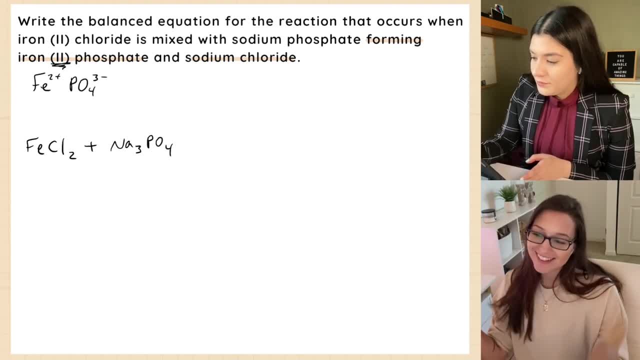 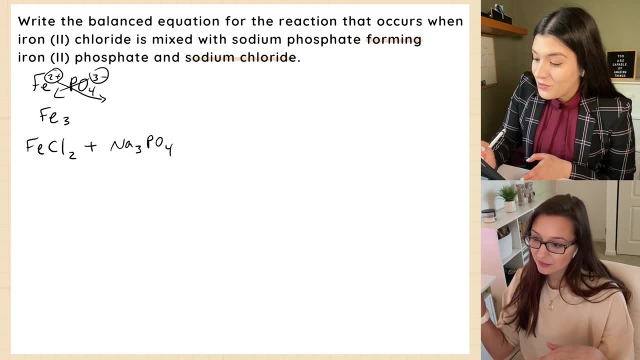 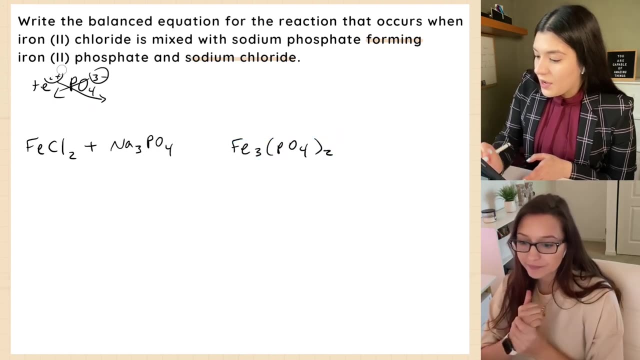 the charge. oh yeah, two pluses, two plus, and then we crisscross, correct. then we crisscross exactly: this two goes here, this three goes here. so this is fe3, and then parentheses po4, with a two on the outside. perfect, i'm going to say. since this was forming, that means that was my product. 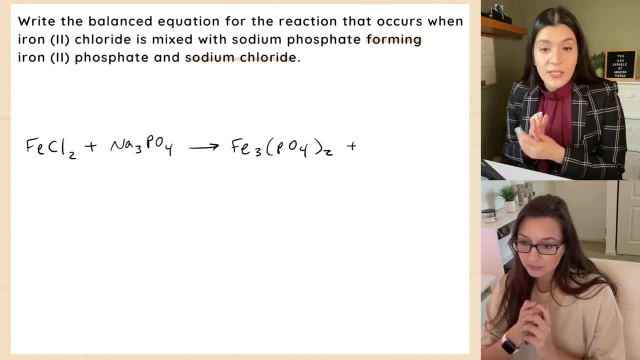 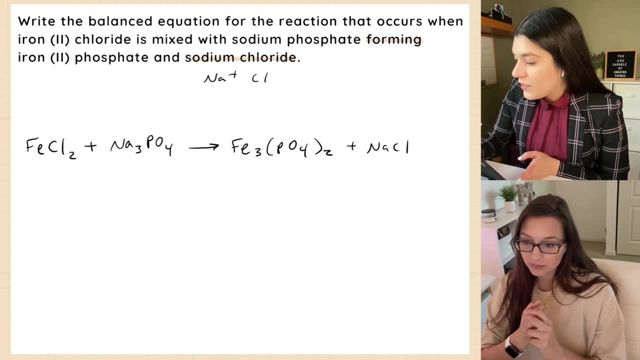 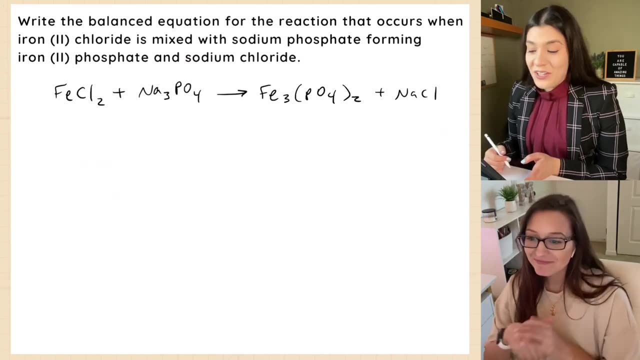 now i'm going to get the second product. so sodium chloride. what's that? n-a-c-l- perfect, easy enough, cool, because n-a has a plus charge, c, l has a minus charge. they're balanced, we're good, okay. next is balancing this actual equation out. so i know i'm combining an insane amount. 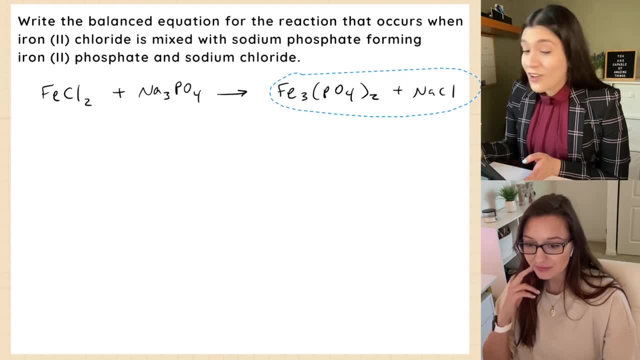 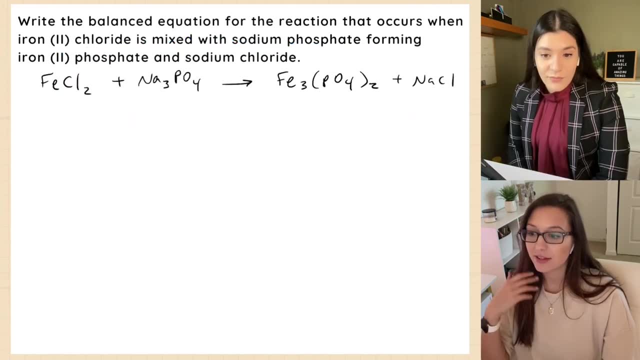 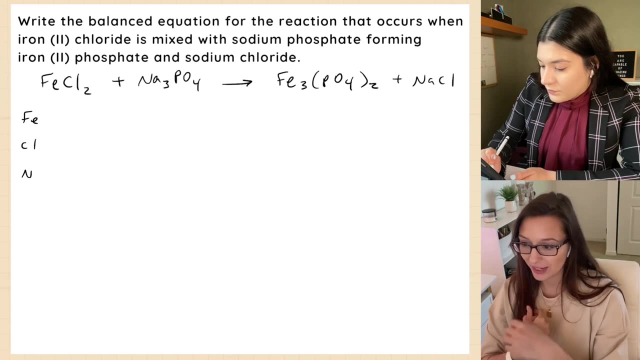 of things all together, but this is good review and this is a common question, So let's just start off with balancing. What's the first thing that we want to do with balancing? Okay, so we have to start out by writing out all of the elements and then we're gonna start balancing. So count how many we. 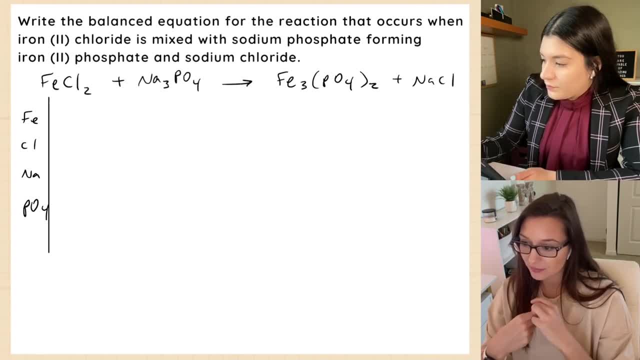 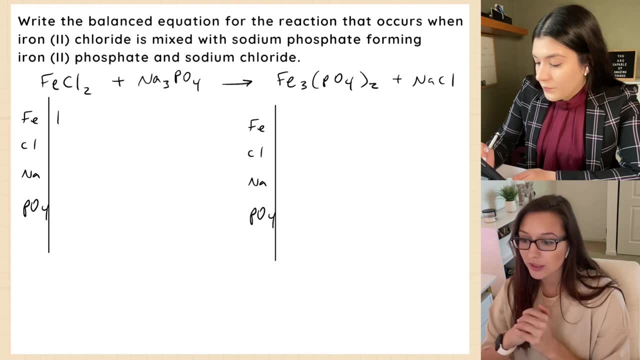 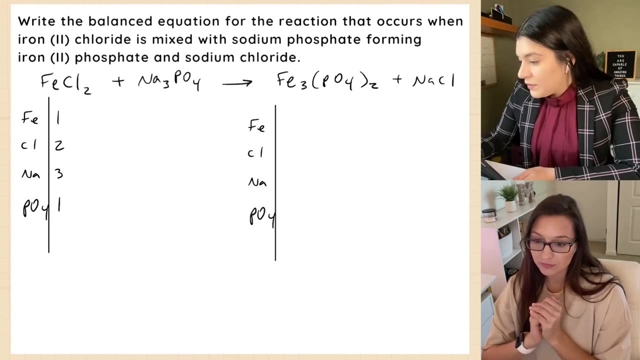 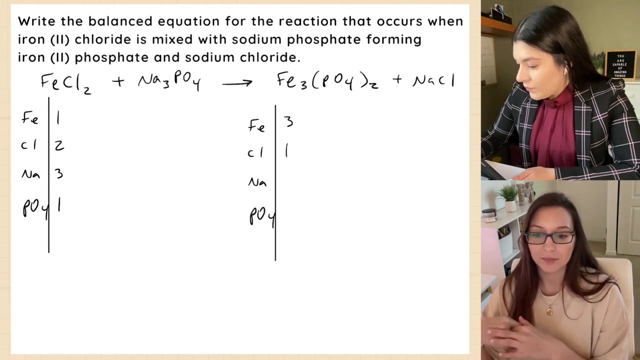 have Perfect, go for it. Okay. so for iron, we have just one, and then there's two chlorines, three sodiums and just one phosphate- Perfect. Next side, And then we have three irons, one chlorine, one sodium and two phosphates- Perfect. Okay, what do? 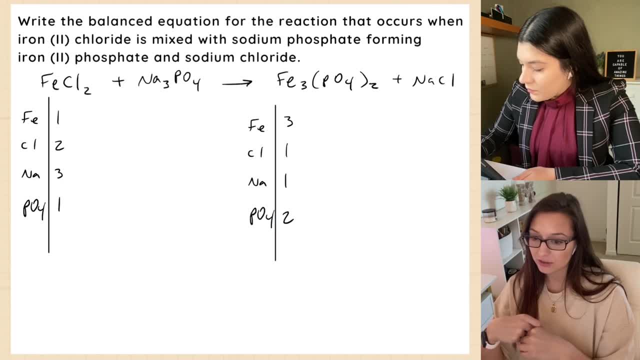 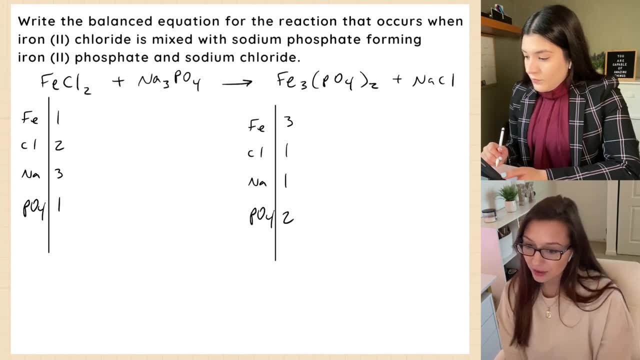 you want to start balancing? Okay, so I guess we can just take it from the top. So for the iron, we need to get to a three. So okay, So for the iron, we need to get to a three, So Okay, so I guess we can just take it from the top. So for the iron, we need to get to a three. So 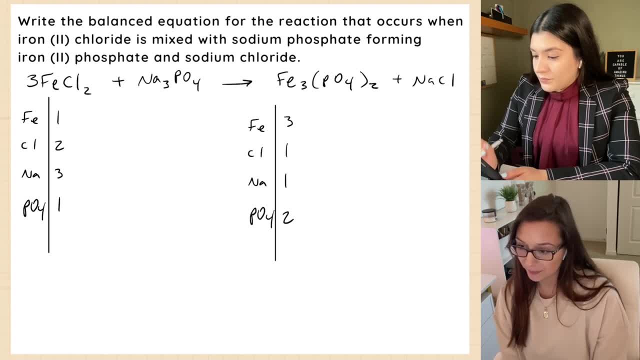 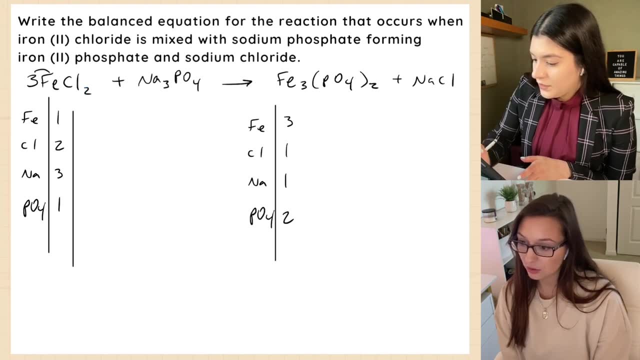 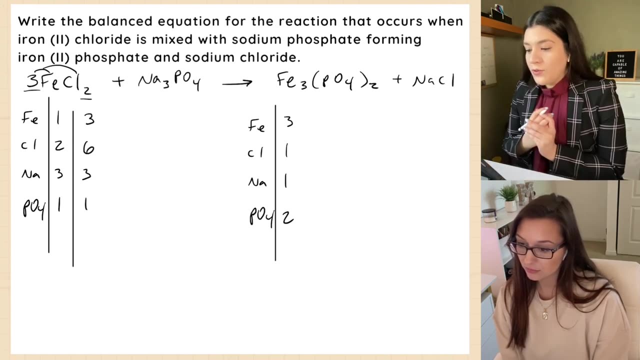 we will put a three in front of it, Yep, And then that multiplies it by both of those, So our new iron has three, and then the chlorine will be six Exactly, And then everything else stayed the same. We didn't change anything, Cool. What's next? 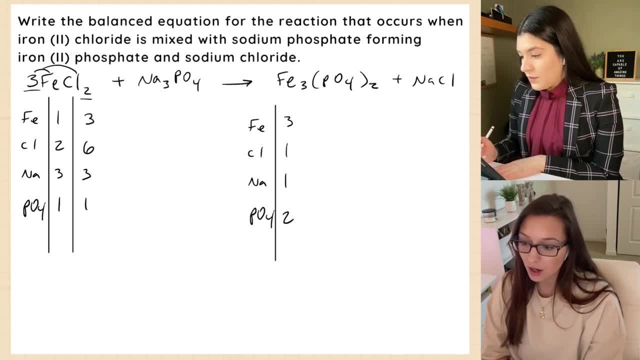 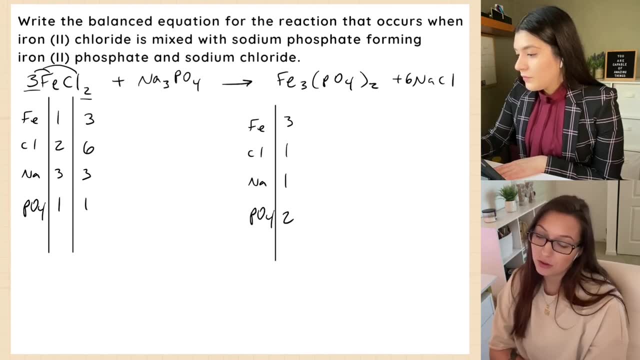 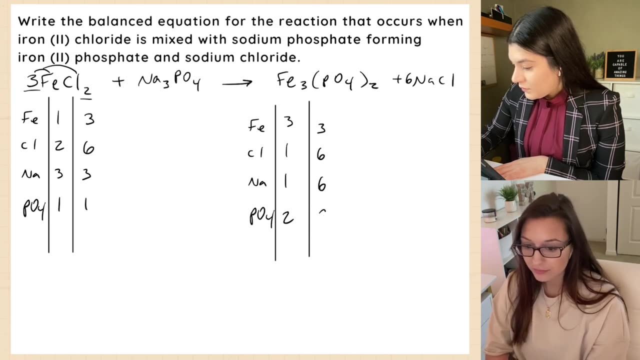 Okay, so next we're gonna do our chlorine, So we need to get to six now. So we'll go over to the product side and multiply the NaCl by six, And so that changes the Na and the Cl to six. Perfect, Okay, keep going. What's next? Uh, and then the sodium. 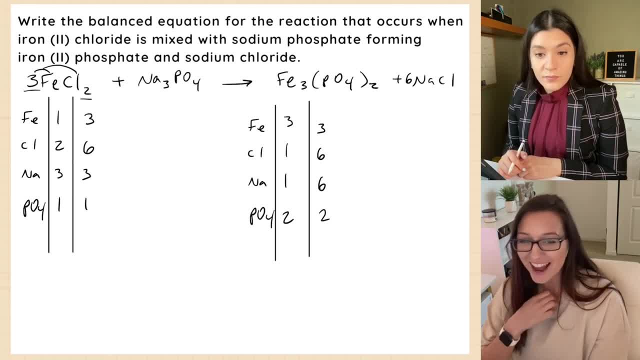 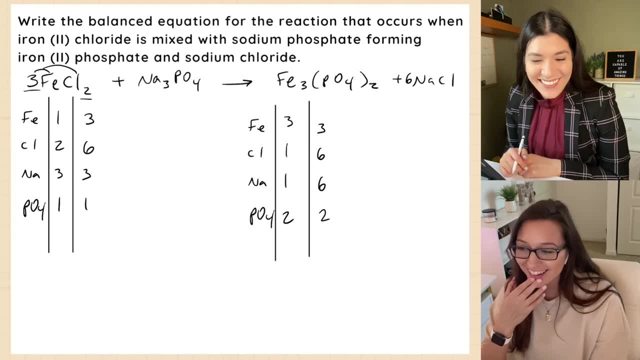 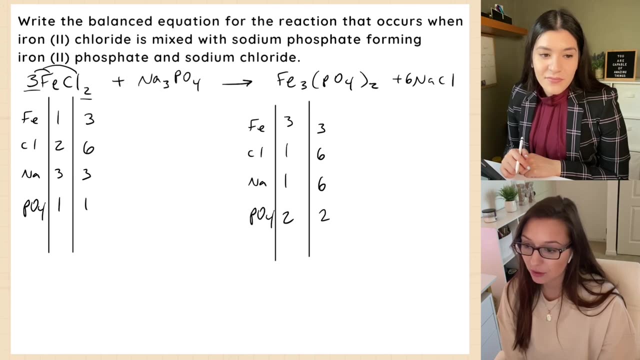 Um, Oh, Okay, Sorry, I just kind of realized, like what happened. Okay, So you can cut that out. Um, okay, So for the sodium we need to get to six. So if we go over to the, So for the sodium we need to get to six. So if we go over to the, 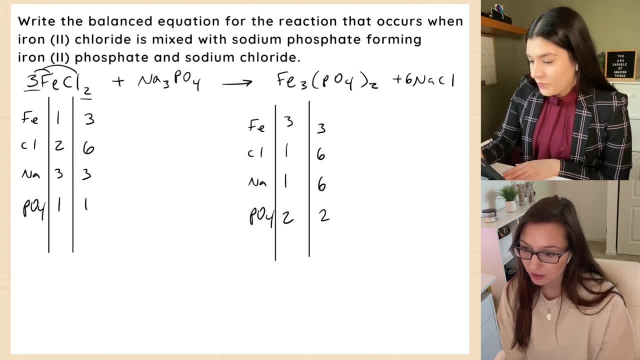 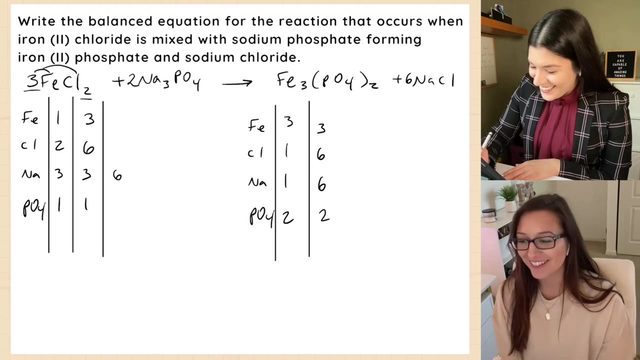 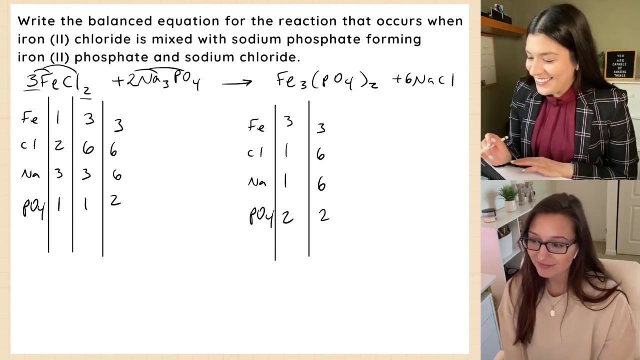 reactant side. we can multiply or put a two in front And um, Good, So that will make the sodium six And it will make the phosphate eight. Wait, no, It will make the phosphate two. That four doesn't go along with it. Good, good, good, You caught yourself, exactly, Good, And then we're balanced. Yay, Okay, So, yay, Cool. So I'm gonna just remove this. We're gonna need this formula. I'm Okay, so, yay, Cool. So I'm gonna just remove this. We're gonna need this formula. I'm going to need this formula. I'm. I'm going to need this formula. I'm. I'm going to need this formula. I'm. 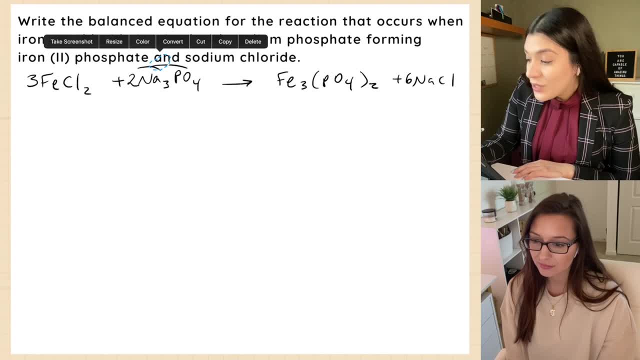 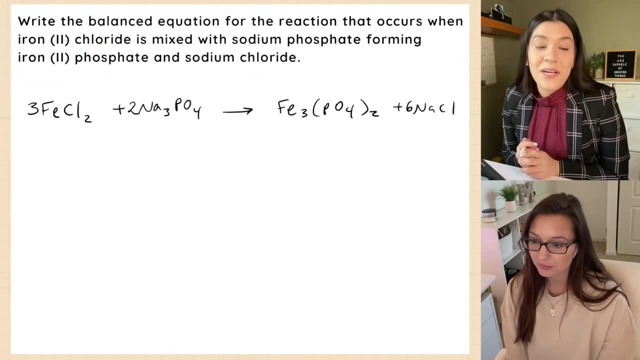 this formula is really important because it is going to help us do the stoichiometry that is part of limiting reactants. So this was just the first step. Definitely, I'd say practice. you know naming compounds, balancing equations, all of this will come up again, as you can tell. 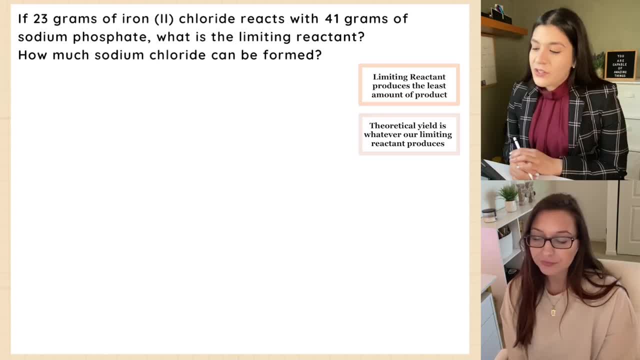 So the next step is to actually find the limiting reactant. So this question is telling us, if 23 grams of iron to chloride reacts with 41 grams of sodium phosphate, what is the limiting reactant? And it also asks how much sodium chloride can be formed. So this is actually asking for two. 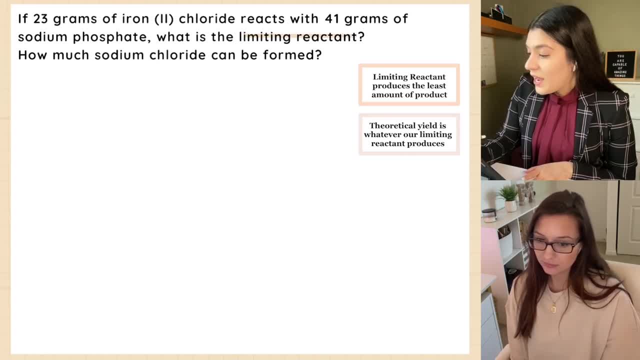 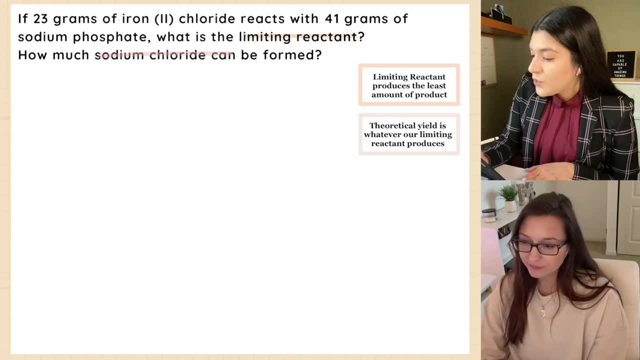 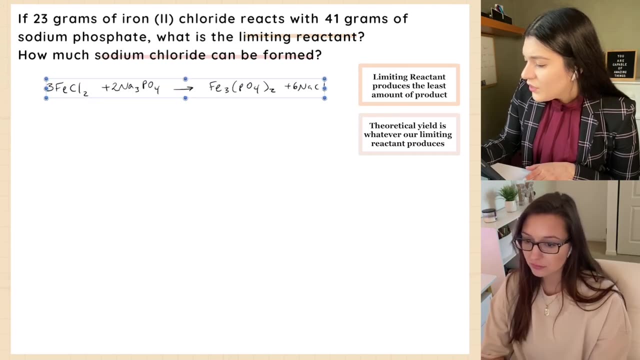 separate things. It's asking for the limiting reactant and it's actually asking for the theoretical yield, by it saying how much sodium chloride can be formed, And I'll explain how I can just tell that that's what it's asking. So, looking back at the formula that we just found, 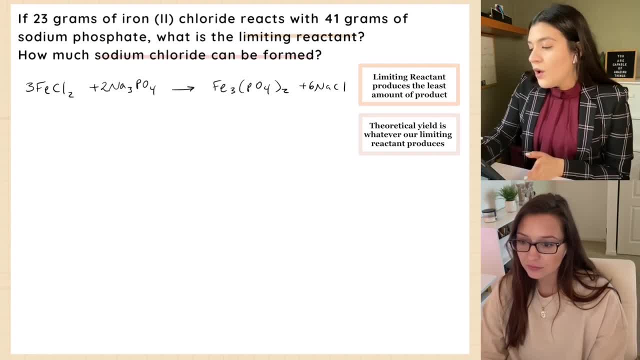 the balance equation that we just found that sodium chloride is a product right, So because we know that that's our product, this is asking us how much kind of like back to the lattes. it's saying: how many lattes can we? 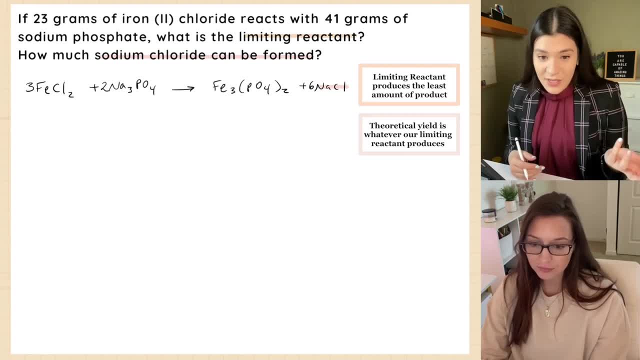 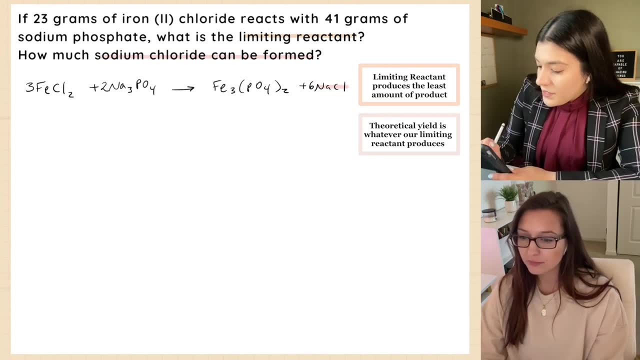 actually make from the limiting reactant. okay, So that's the concept here. So the first thing you want to do is to just find the limiting reactant. How we do that is we're going to take the grams of each reactant that's given, and we're actually we have two reactants, right? 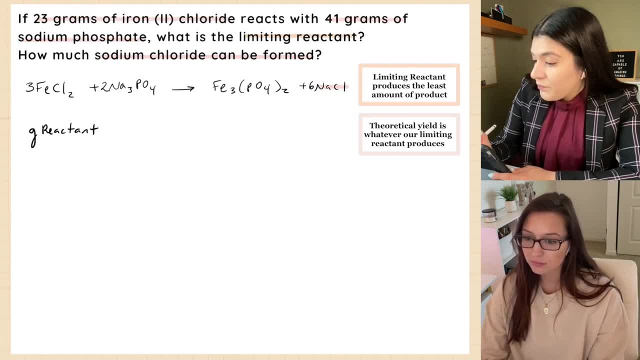 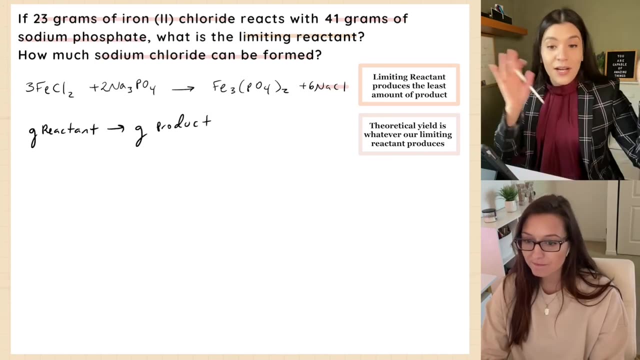 And the mass of two different reactants And then we're going to make our way to the grams of the product. So this is going to be a long process and it's going to be a bit more of stoichiometry, So we can't just magically go from the grams of a reactant to the grams of. 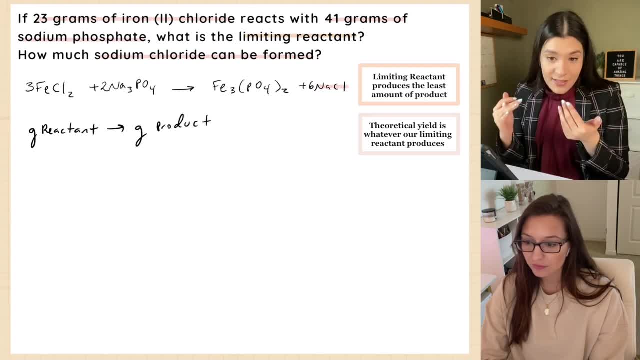 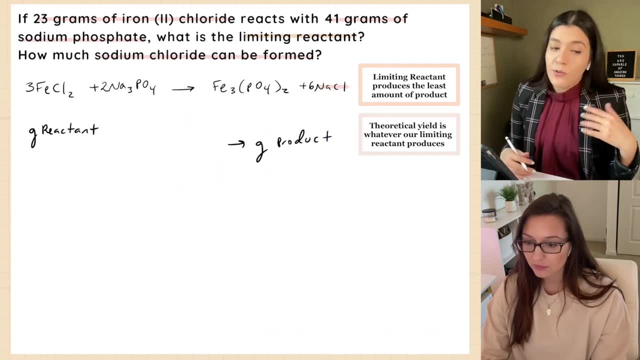 our product right. There's no one conversion factor that can take us there, So instead we have to go through kind of a series of steps, And this is what it's always going to be whenever we're going from the grams of our reactant to the grams of our product. 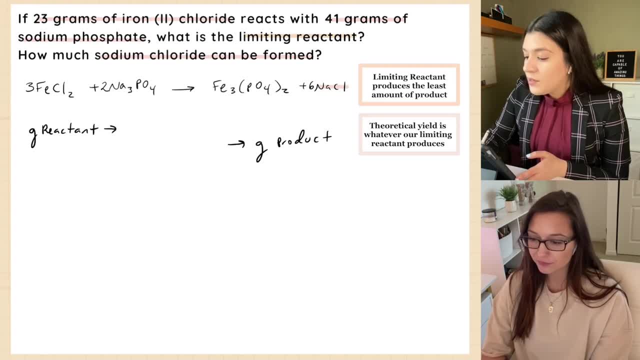 So we're always going to go from our grams of our reactant to the moles of our reactant, Then we're going to get to the moles of our product And then, lastly, we'll be able to get to the grams. Let me just make some room. So is this the same every single time? 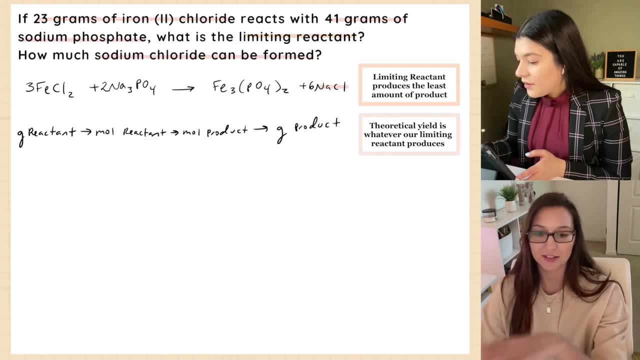 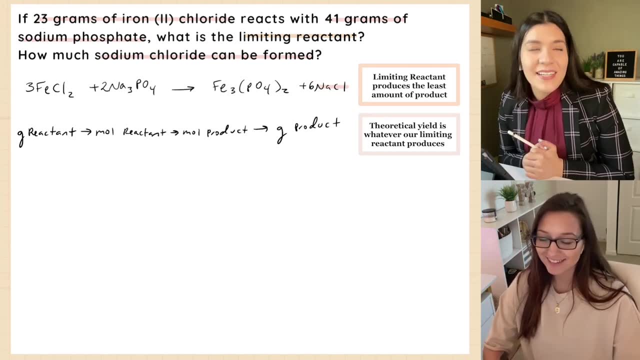 Yes, So I can just like kind of memorize this product And then it'll be for every limiting reactant, or I never want to say memorize, I always want you to understand, Yeah, because, But like the steps will be the same, right. 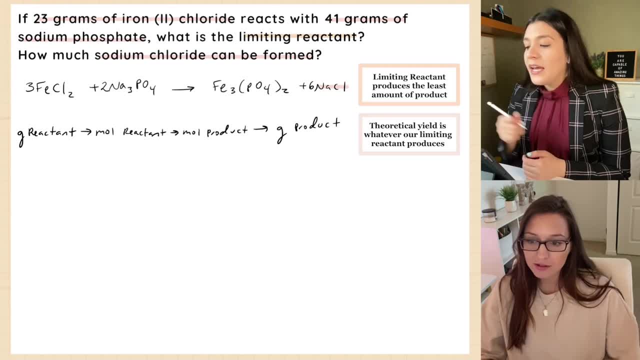 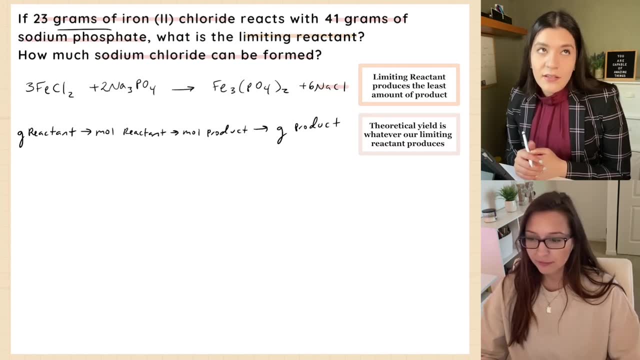 The steps should be the same. Correct. The steps should be the same if you're given grams. So if you're starting off with grams of your reactant and it's asking you know you define, like how much of your product is formed, then yes, you'll go to grams of your product. However, if it starts 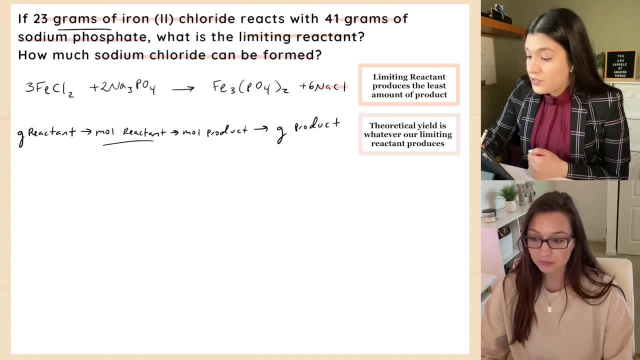 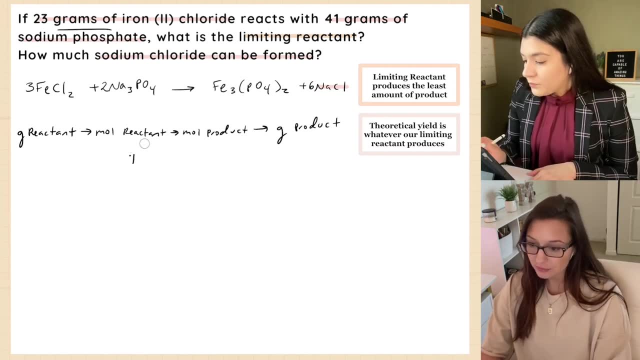 with the moles of your reactant. then you would have just like skipped the first step and you would have started here. Okay, I see, Yeah, Yeah, Cool. So in this case, I'm actually going to go. I'm just going to apply this to everything that we have Instead of our, so our first reactant. 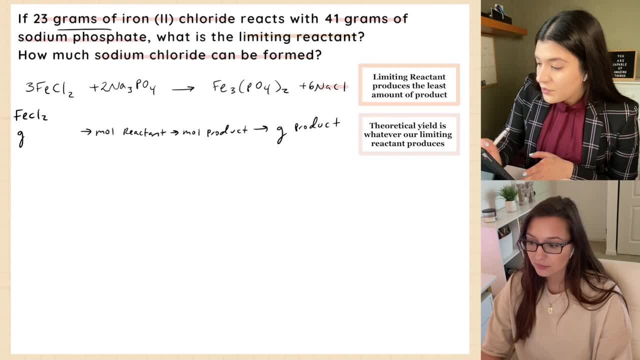 I'm going to do this for our first reactant, which is, we said, iron chloride, And I do like just putting whatever reactant that I'm actually like doing this for on top, just to separate everything. You'll see why in a second, But I'm actually going from the grams of my first reactant to then. 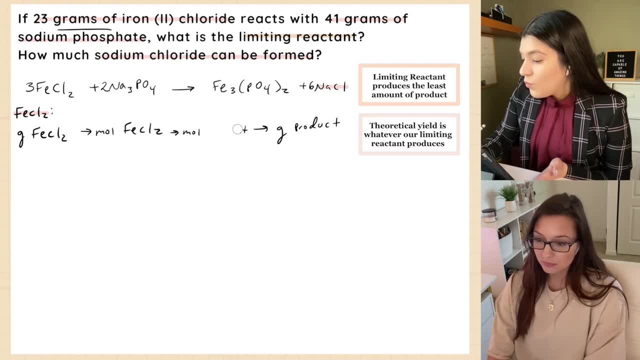 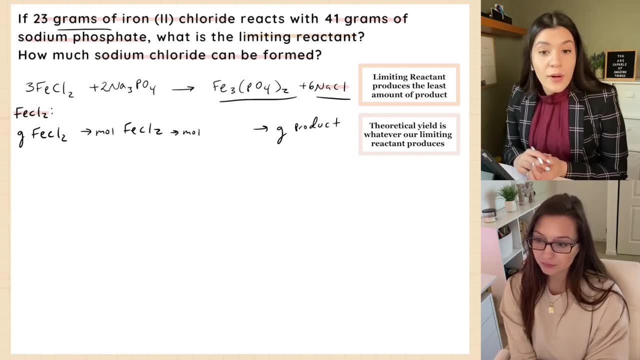 the moles of my first reactant to the moles of the product. And here we have two different products. If you weren't told you know how much sodium chloride can be formed, then it wouldn't have mattered which product you would have chosen. So as long as both of the reactants that you're 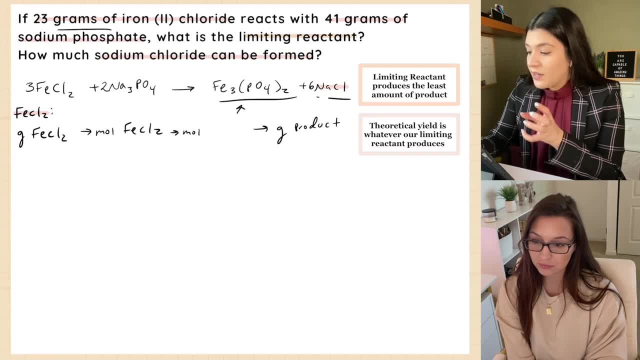 taking go to the same product. So meaning, as long as you just like commit to iron, you know phosphate, picking that one for both of the reactants, you know the process, then that would work. Does that make sense? Yes, Kind of Okay, I can reiterate it once. 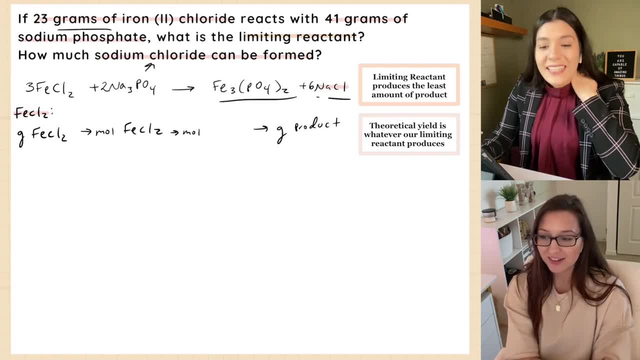 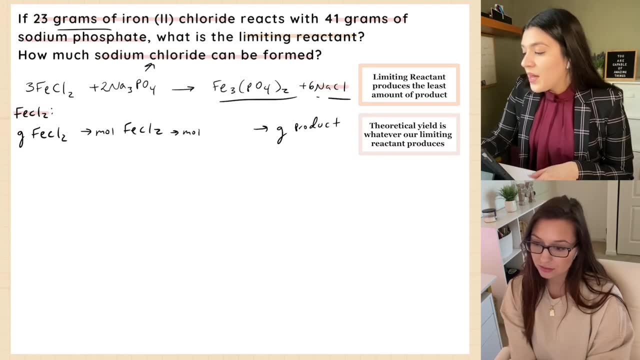 once you see the whole stuff, Yeah, Once I see the next one. but I think I get what you're saying. Yes, Okay, But but because this already asked me, you know how much sodium chloride am I going to form? I know that the product that they want is sodium chloride, So I'm actually going to sodium. 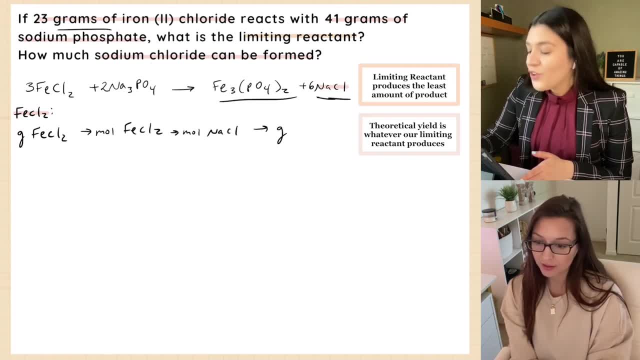 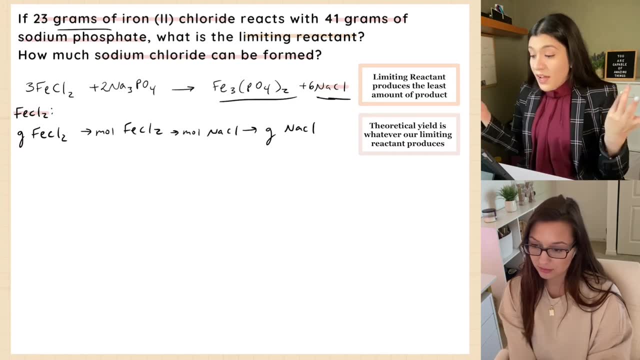 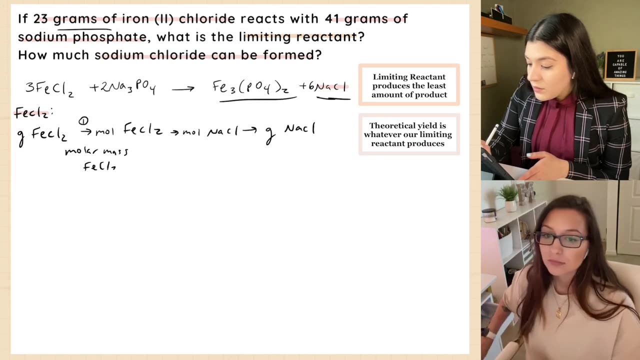 chloride, So we'll use that for both. So right, Okay, Correct, Cool, So awesome. I'm just going to plug everything in. The first conversion factor that we're going to use is going to be the molar mass of iron chloride, And let me just set this up So. 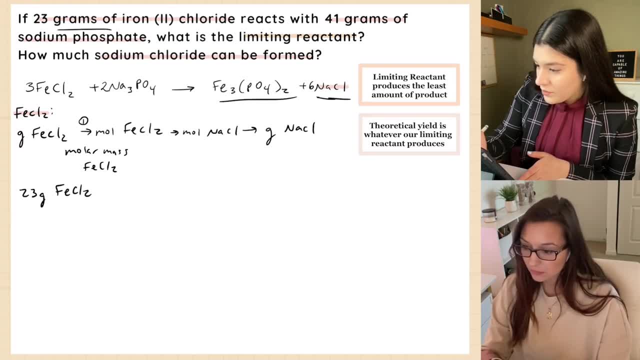 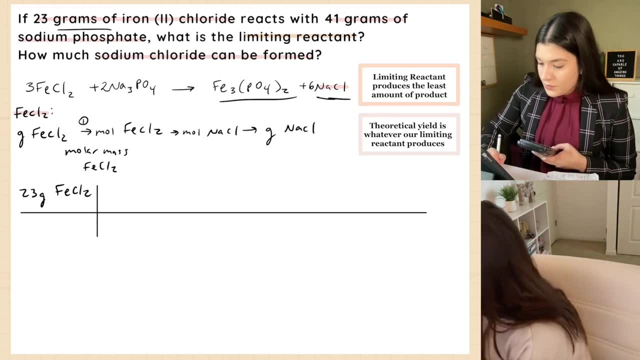 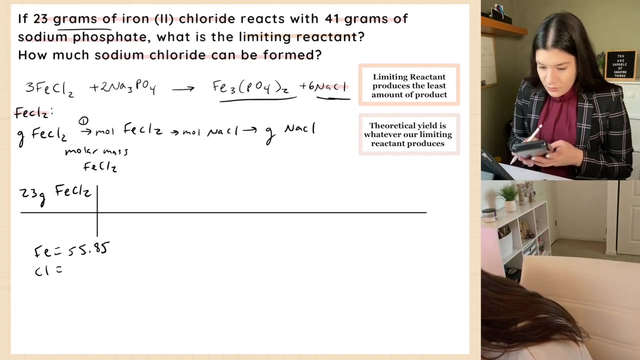 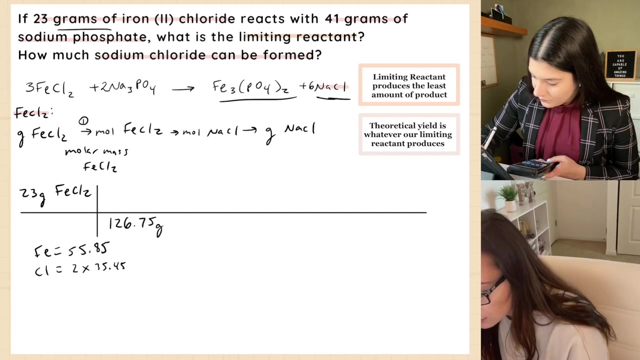 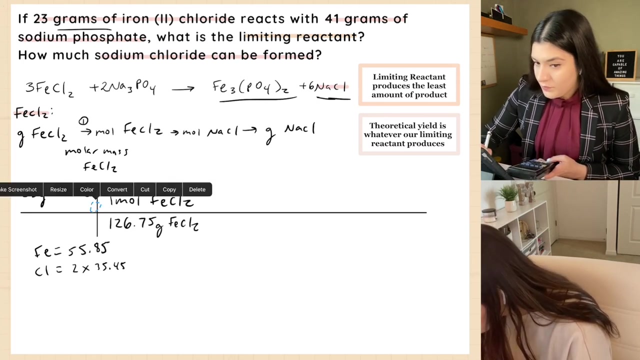 23 grams. I haven't found with the masses. So if you want to do that as well, just going to do that here? Cool, Just 35.45 times two, Okay, And then all those added right. I need to get a giant periodic table because whenever I'm looking at like the little teeny numbers on this, it's so hard to see. 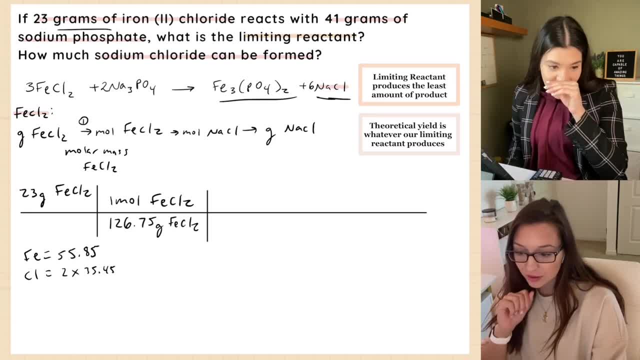 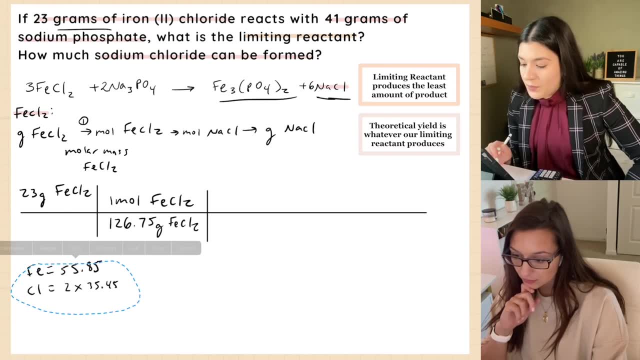 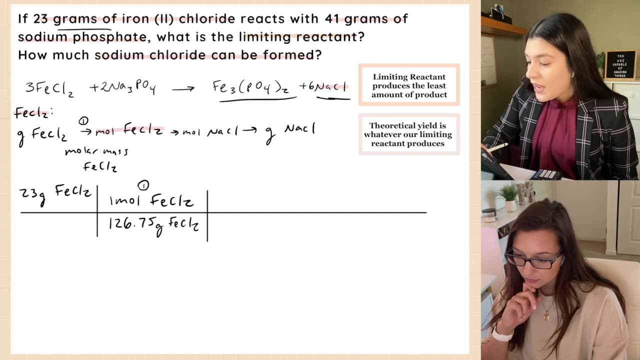 Right, I got the molar mass. So I know you know how to do molar mass, but um, cool, So that's what we would get for the first part. Um, after we added all the mass, individual masses of our elements together. next, uh, that was our first conversion factor. Now that I'm here at moles of my reactant. 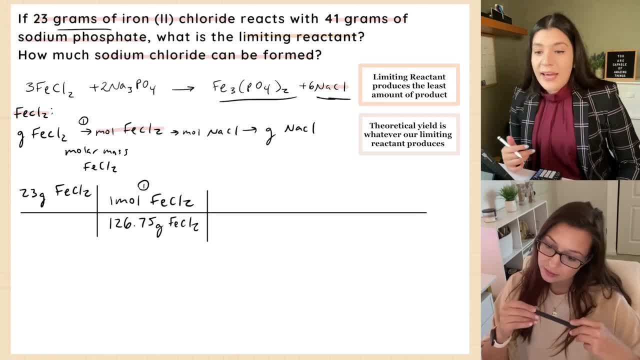 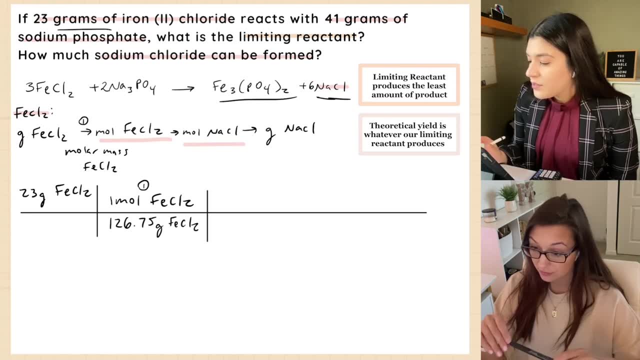 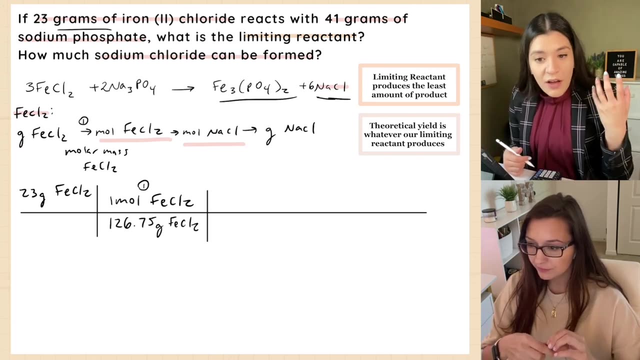 Okay, Now I have to do a multiple ratio and something to kind of just note. So this is stoichiometry, where this, this portion, basically like how you know to do multiple ratio- is the fact that you want to change the compound We have. we start off with one compound, which is iron chloride. 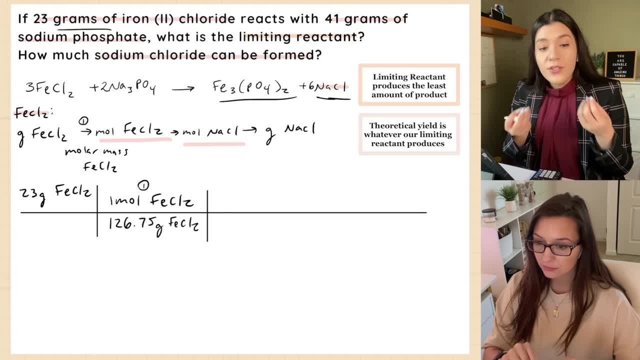 And now we want to change the compound to sodium chloride. So to be able to do that, you need to use a multiple ratio from the balanced equation, And that's why it's so important. So I would look at the coefficients in front of whatever I'm looking for. 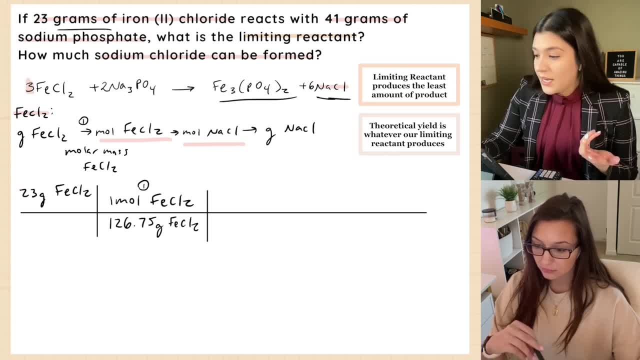 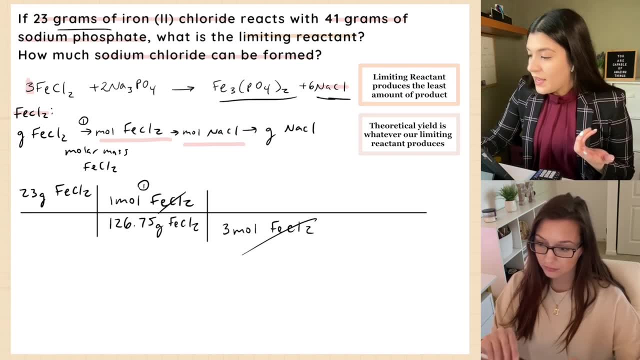 So the moles of iron chloride are three and I'm going to place that on the bottom. So three moles of iron chloride, just so these units can cancel. And then next I'm going to look at sodium chloride and the coefficient in front, which 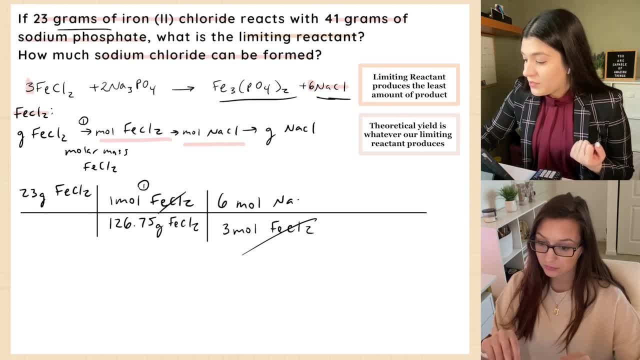 is six. So that's where I'm taking these numbers from. is from the balanced equation Make sense? Yeah, And then, now that we're here, we're at this step, We're at moles of NACL. I'm going to again. 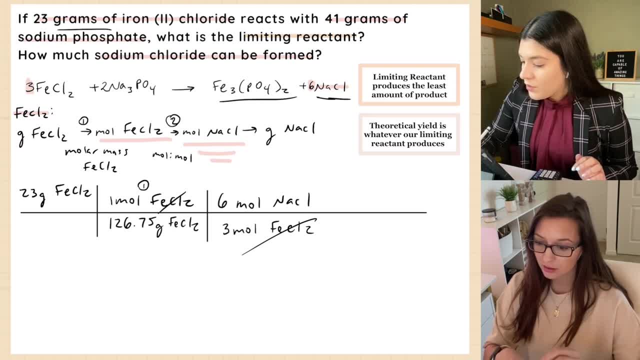 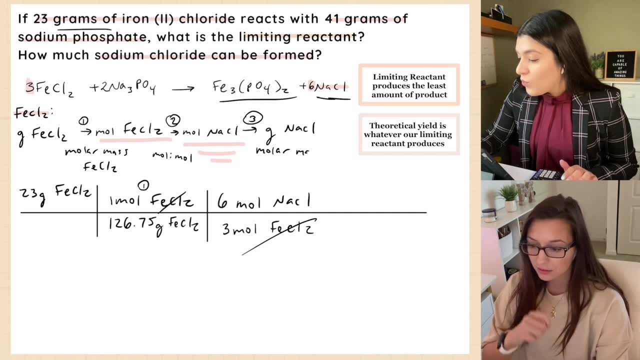 So I'm just going to just show this real quick that this was a multiple ratio. And then the third conversion factor is just using the molar mass. again, Whenever we're going from moles to grams or grams to moles, we use the molar mass of whatever. 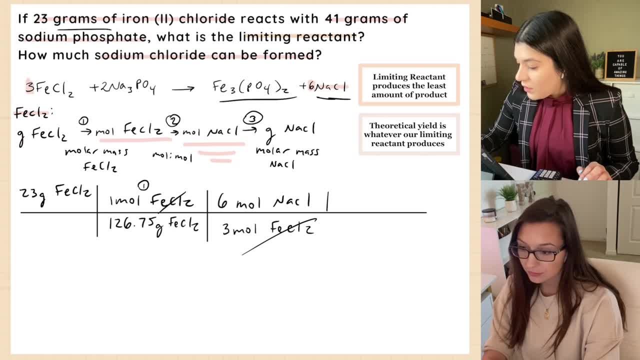 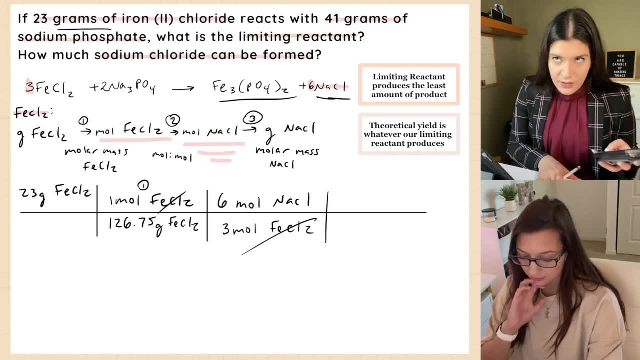 compound we have. So this, in this case it's NACL. So I'm going to just find this again, adding up everything, all the masses of chlorine and sodium. I think sodium is twenty two point nine nine. Yeah, So if you're just like, I'm just 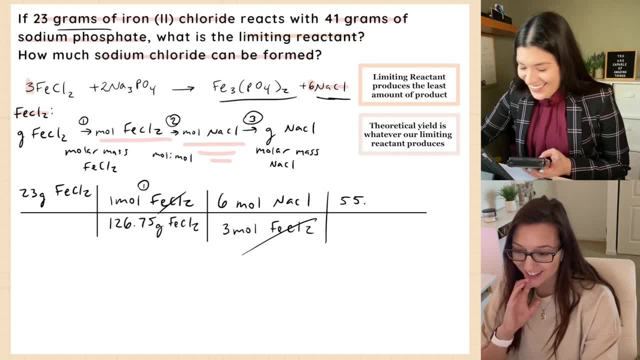 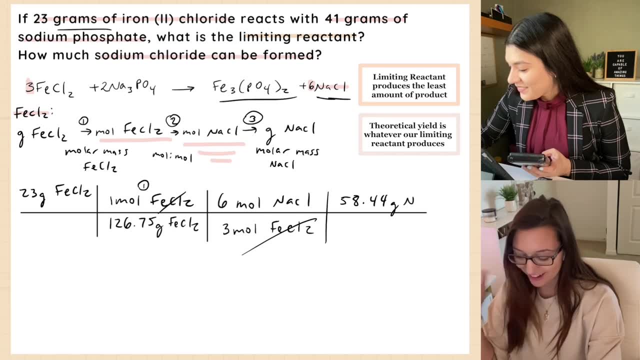 I'm just going to, just going to let you do your thing. I, yeah, I'm writing down like the steps, because I know you're going to give me practice problems, That's true. I'm just trying to write down like, OK, first step, molar mass. second step: the ratio. 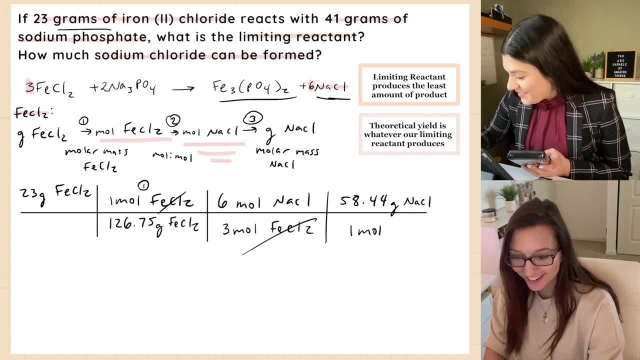 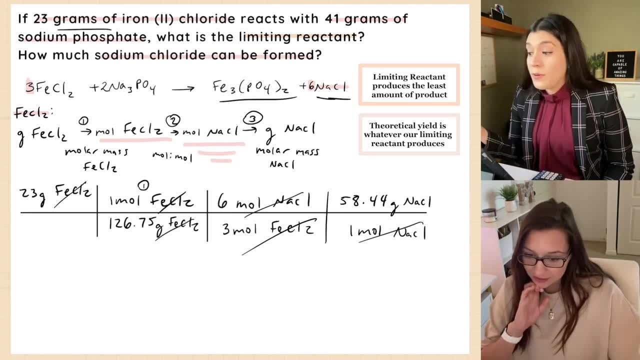 Yes, Yes, that's totally fine. I'm glad you're doing that NACL Cool. And then you'll see that all of our units cancel to give us what we want, which is the mass of our product. So now I'm just going to multiply straight across. 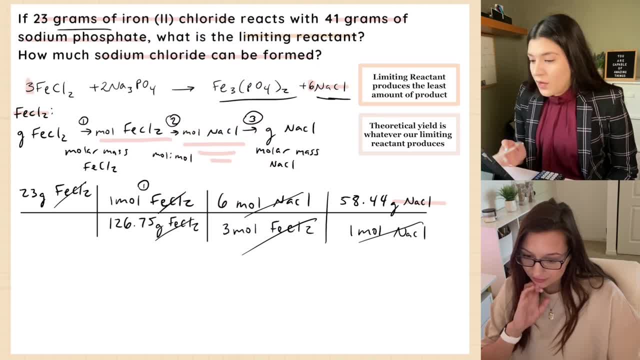 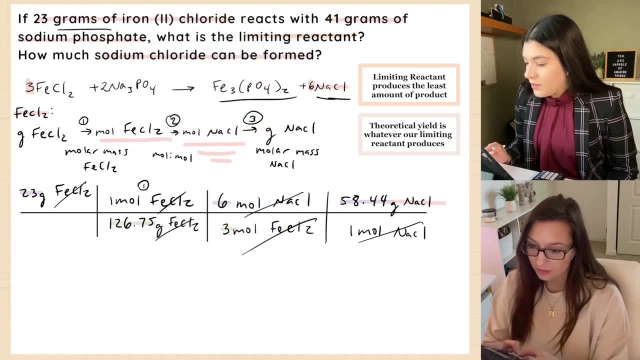 And then divide by, you know by the, the bottom. So I'm going to multiply twenty three times, six times this value, And then I'm also going to divide by by these two multiply. So Let's see what this gives us. 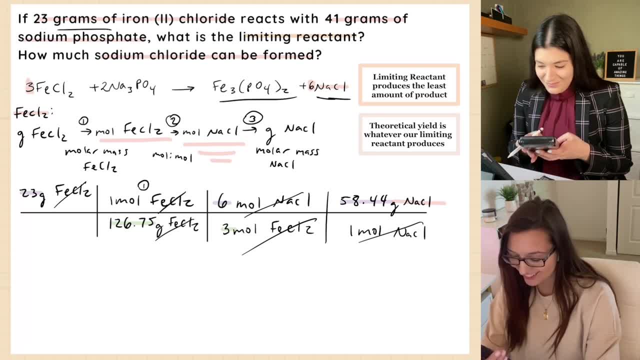 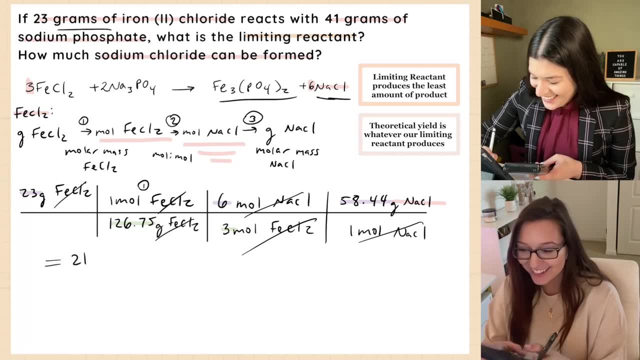 I haven't used the calculator in a while because everything else we've been doing hasn't really needed it. Lewis structures- Yeah, Lewis structures. Those are a good time. Sadly it's over now. I know I have to do real math again. 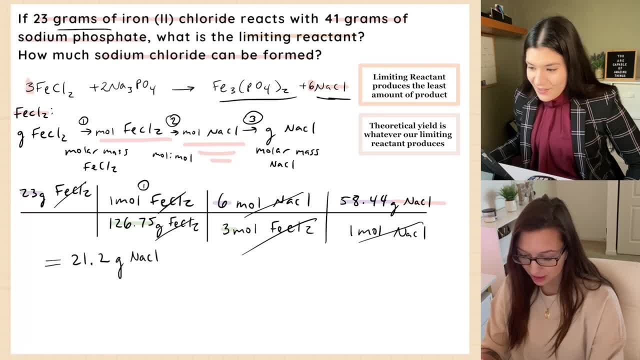 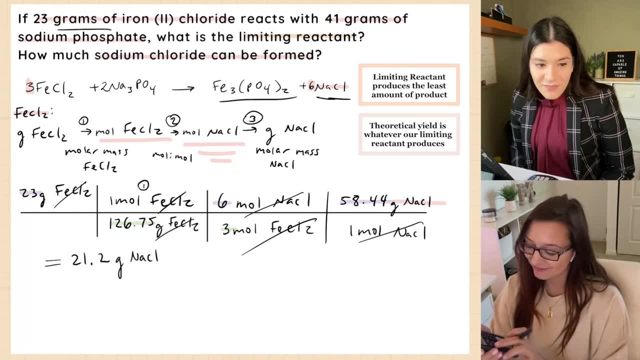 OK, let me know if you got this. I'm still calculating the bottom. Now I'm dividing OK. OK, Um, twenty two. we're twenty one point two. Yeah, cool, So I would say, oh, and one thing I'm also going to mention is just the fact that I'm 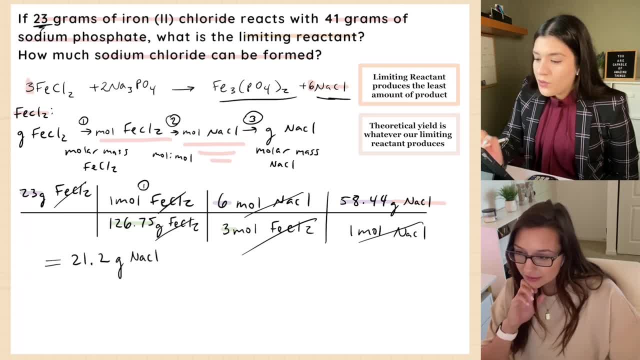 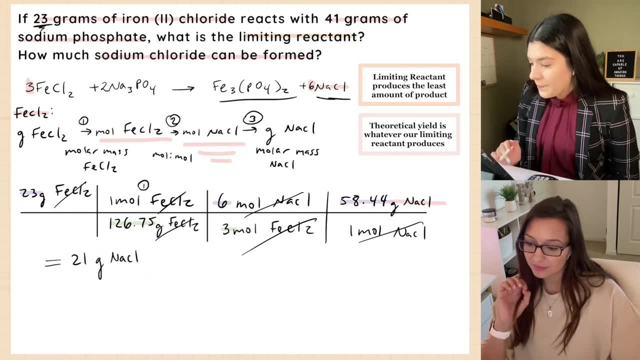 actually even going to round this down a little bit more. This is only two sig figs, So I only want two sig figs. So I'm just going to say this is twenty one. OK, I see, Yeah, So OK, that's. that's the first part where I'm saying: all right, this first reactant. 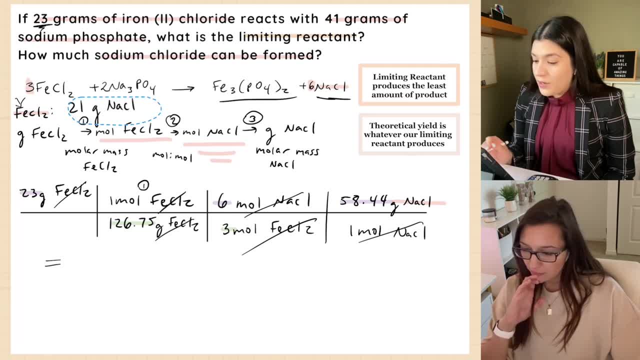 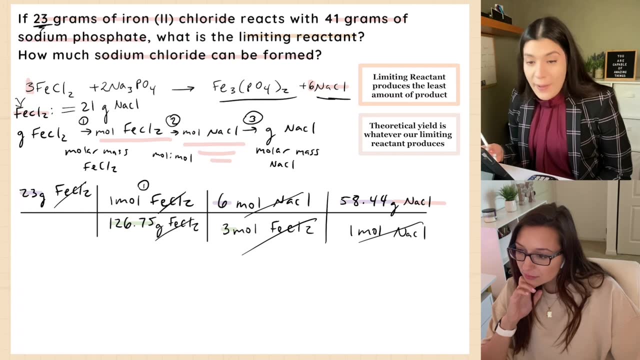 this first reactant here produced twenty one grams of here. I want to put them like all together. I'm just going to put it over here. OK, This first reactant produced twenty one grams of my product. OK, And I'm going to do this all over again. 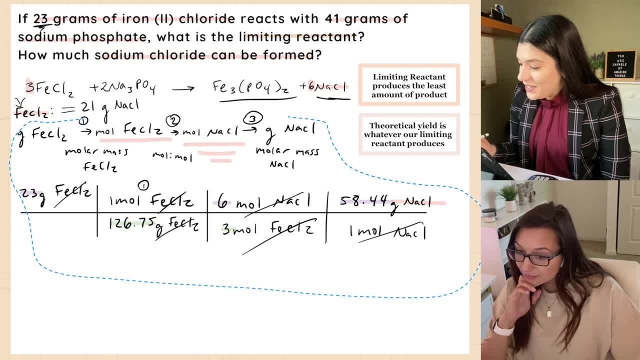 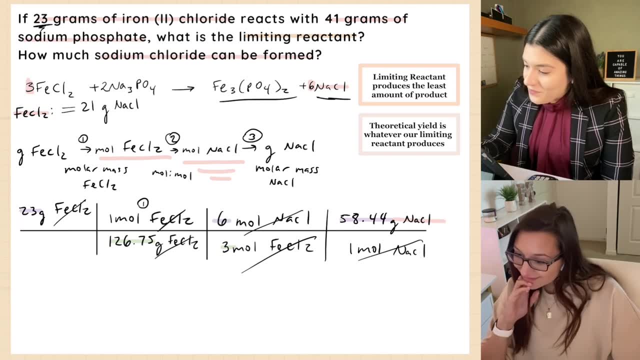 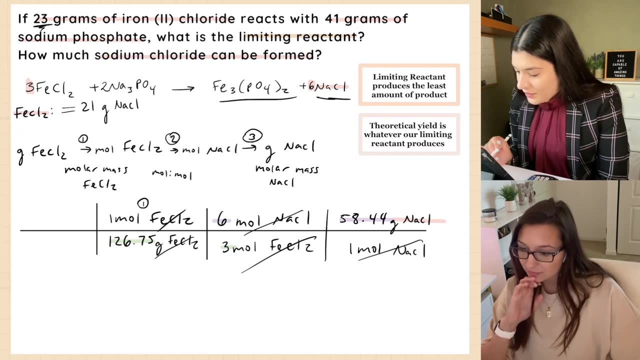 OK, So let's redo this for the second reactant And you do this for each reactant, So luckily there's only two and typically there's only two. But all right, I'm going to do this again and I'm just going to replace everything that I need. 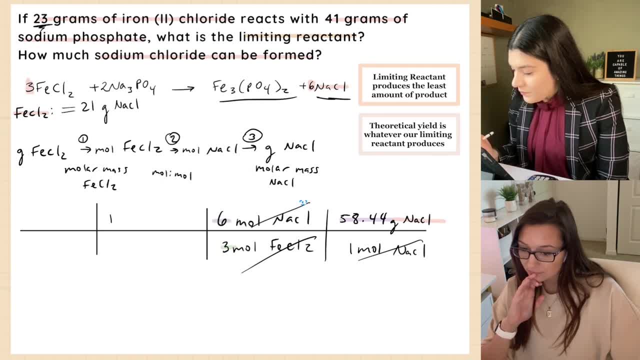 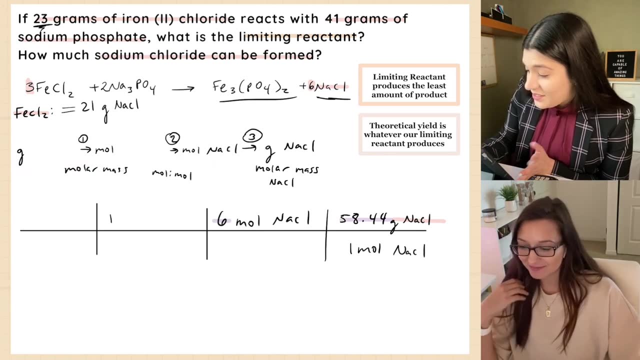 OK, Come on, All right. So the next reactant- if I can delete things fast enough- the next reactant that we're going to do this for and you're really going to see this same sort of setup every single time. 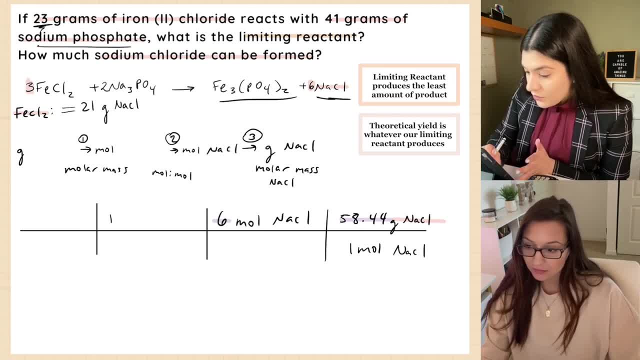 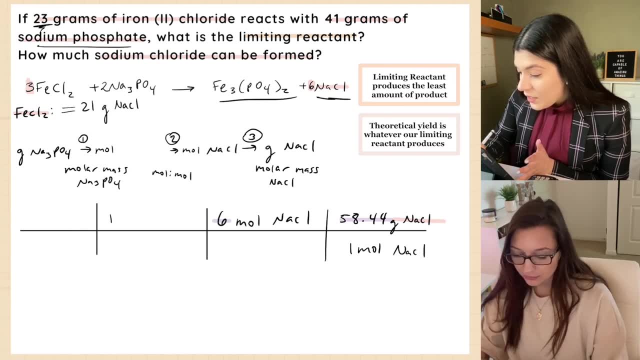 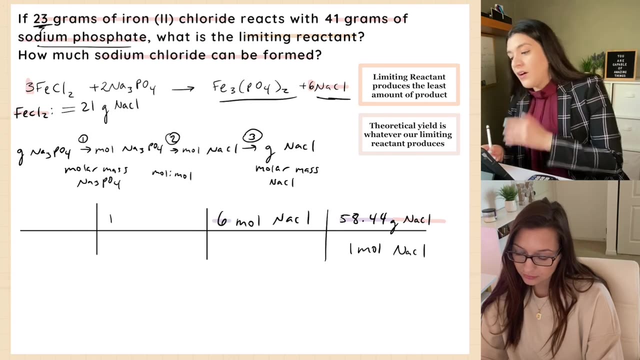 The next reactant is our sodium phosphate, So I need the grams of sodium phosphate. I'm then going to use the molar mass of sodium phosphate to then get to the moles of sodium phosphate, And then it's the same process again: mole to mole ratio to change the compound, and then 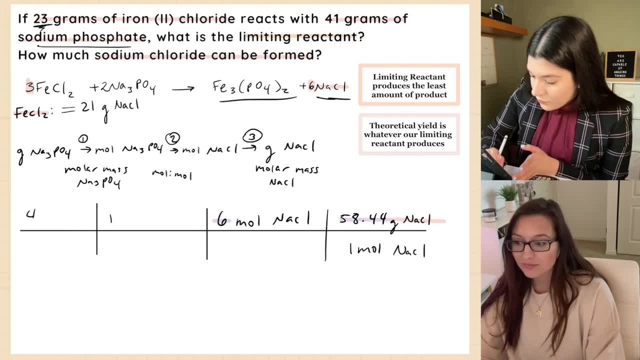 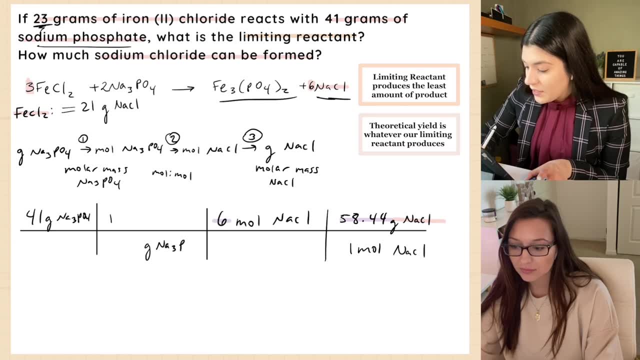 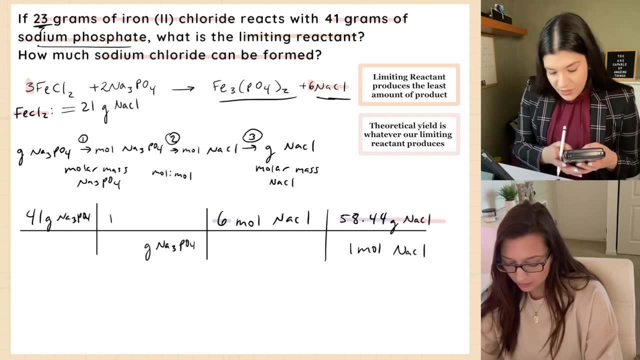 our mass of sodium phosphate, Sodium chloride. So I'm going to start off with the 41 grams of sodium phosphate. I now need the molar mass of sodium phosphate. So I'm going to do this real quick. add everything up. This is 22.99 times three plus phosphate's mass, which is 30.97 plus four times 16.. 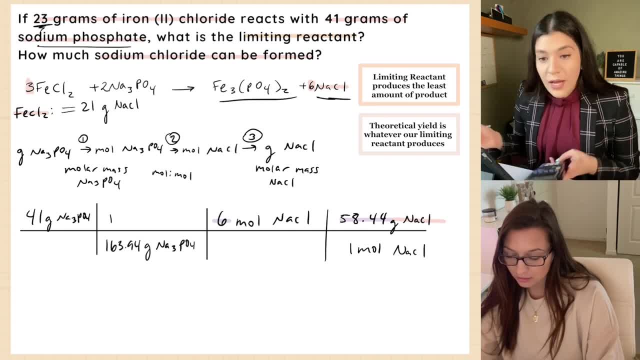 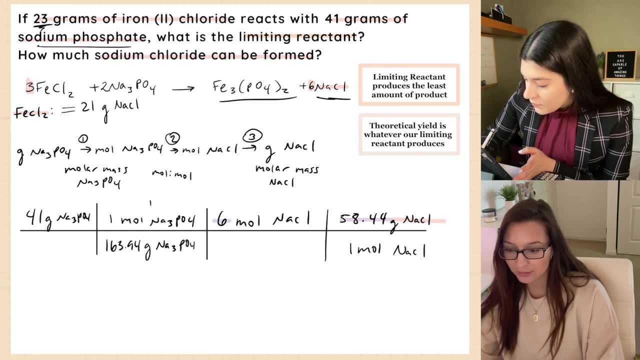 So I get 163.94 grams of sodium phosphate. That's the molar mass. That's the molar mass, And then for every one mole of sodium phosphate. And when you're doing the phosphate molar mass, you're just doing like phosphorus and 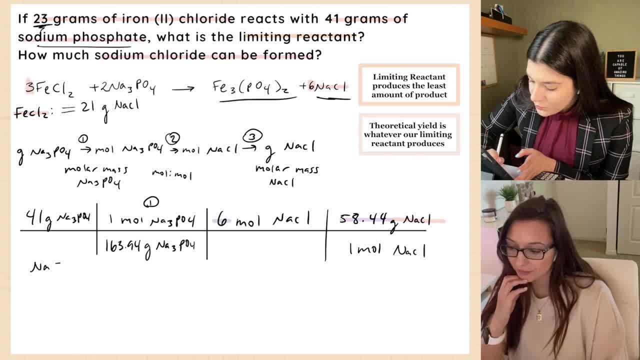 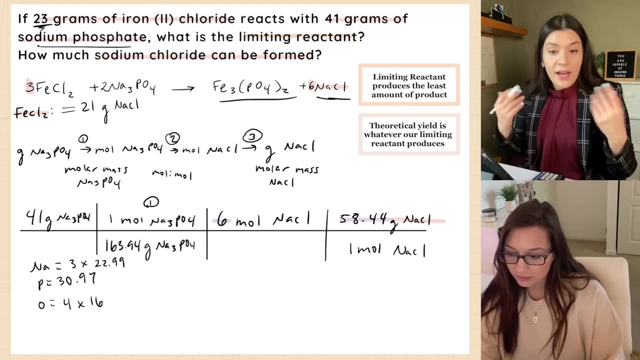 then four oxygens. Correct, Yeah, I'm multiplying everything. So I just want to show it just for everyone as well. I'm multiplying. you know, every single subscript with the element Phosphorus was 30.97, and then oxygen was four times that- 16, and then multiply, add everything. 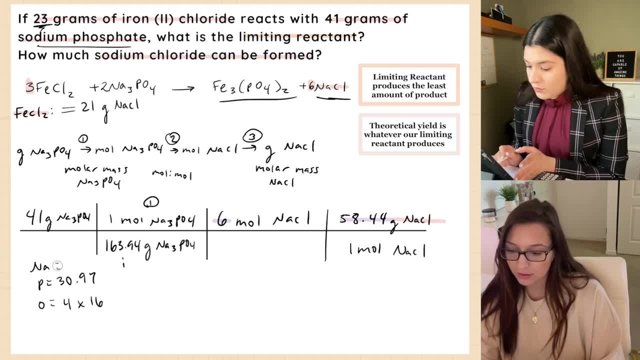 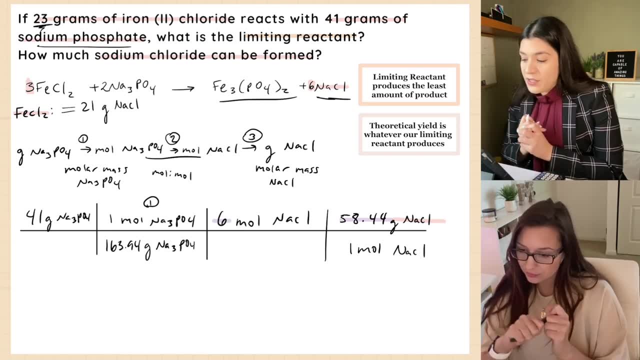 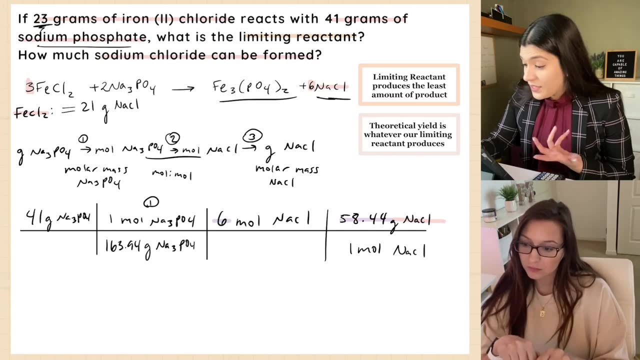 together And then that gave me that 163.94.. Yes, Okay, Cool, Cool. Next. So we're going to be at this step where we're changing this to moles of sodium chloride, So I need to use the coefficients again and I'm going to look back and see: all right. 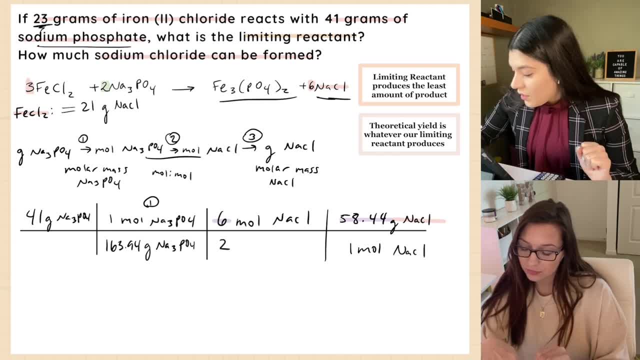 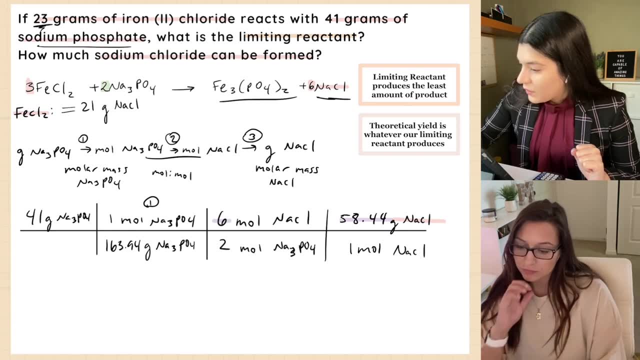 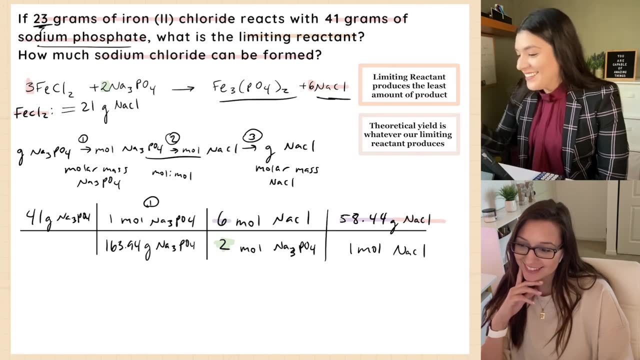 sodium phosphate has a two coefficient, So this is two moles of sodium phosphate. I just used again the periodic table. Okay, So the periodic table, actually periodic table. I just used again the balanced equation. Goodness, Yes. And next, this is basically the same exact setup, right? 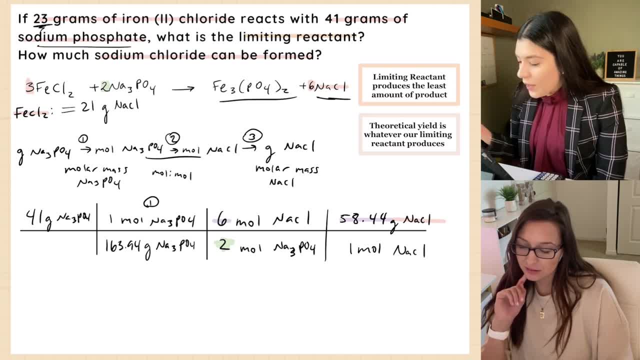 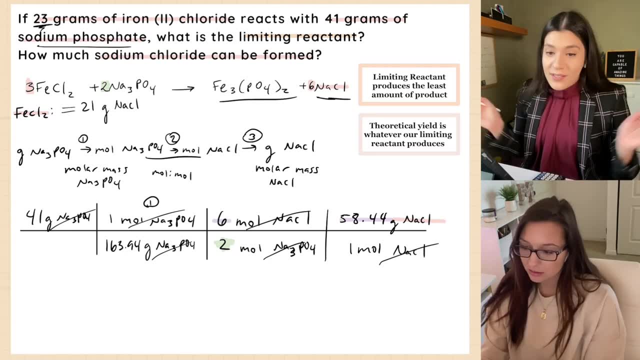 We're going to go again to grams of NaCl. So okay, I see that grams and grams cancel moles, moles cancel moles again, and we're left with what we want. So same process. I'm going to multiply straight across divide. 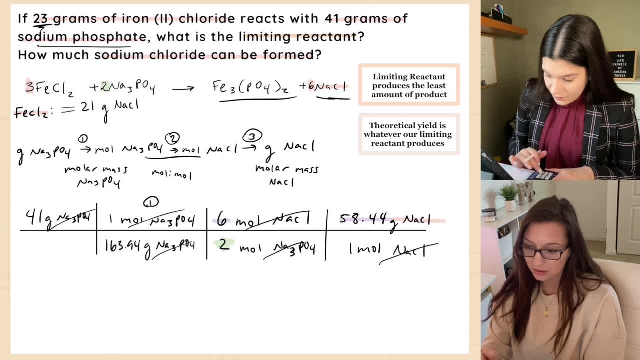 Okay, And let's see what this gives us. Okay, And then I would. I'm going to round to two sig figs, So I got 43.8, but I'm going to round up to 44 grams of sodium chloride. 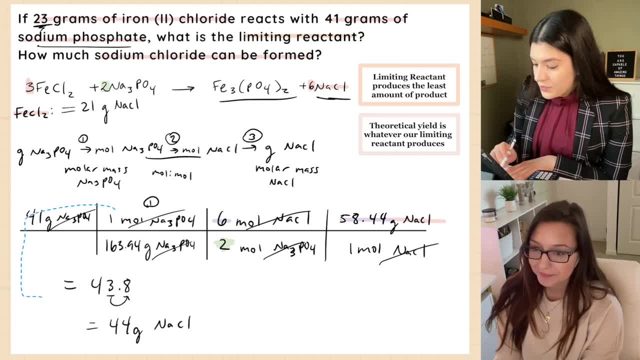 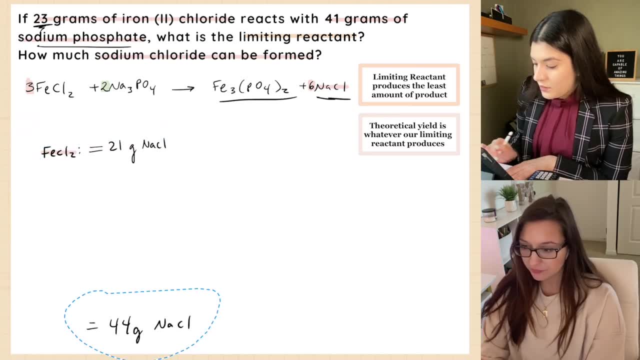 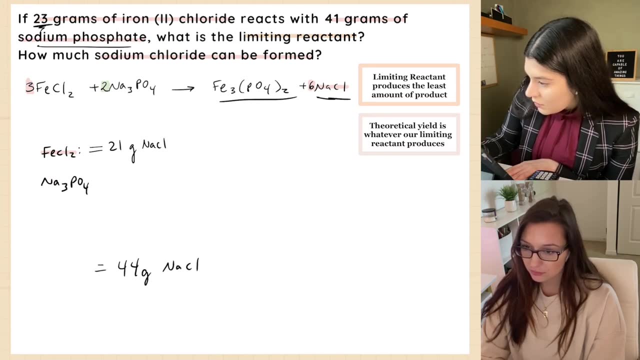 Perfect, That's what I got. So perfect, Cool. So I'm going to just kind of remove all of this and just show you. I'm going to separate this And then let me put that. Our second, Our second reactant produced this: 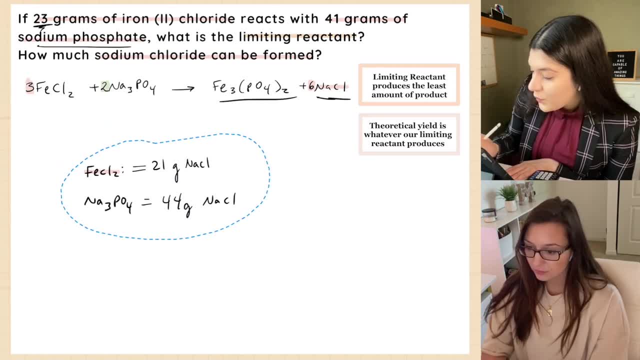 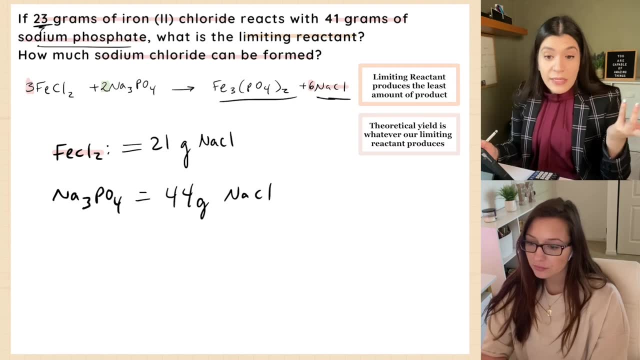 So this is both of our reactants and how much product they actually produced. Now the reason why I like to separate this at the end, or even in the beginning, is because, after you do all this math, typically I've seen students say, oh, the limiting reactant. 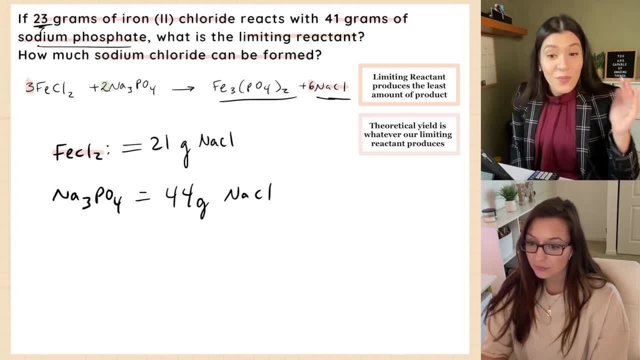 is NaCl And it's like: no, no, no, that's the product. right, That's not a reactant And it's just because you forgot kind of what you were doing in this. you got lost in this whole process. 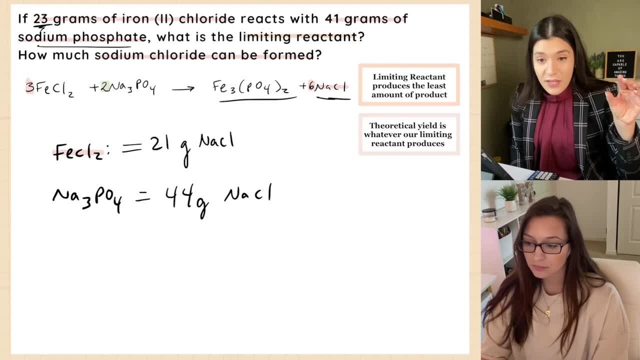 So it's important to know. all right, this is the reactant that I started with, And then I'm I'm picking from these two to say whether or not they're a limiting reactant or not, because they are reactants. 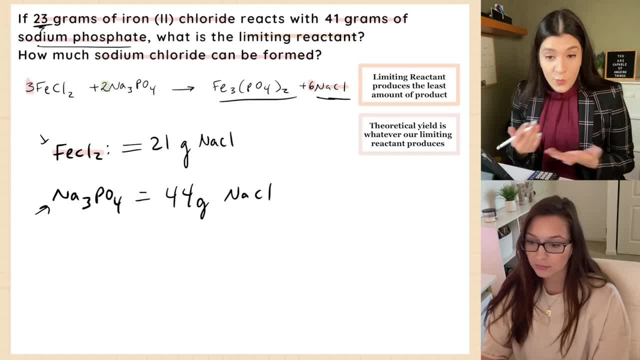 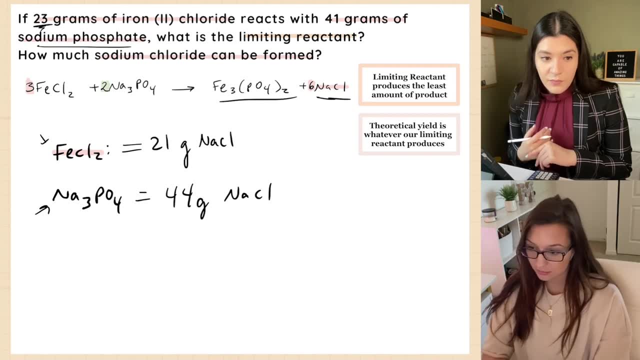 So we said that the limiting reactant produces the least amount of product. So which one of these reactants produce the least amount of product? The first one? Yes, So this one is the NaCl. This one is the limiting reactant because it produced the least amount of product. 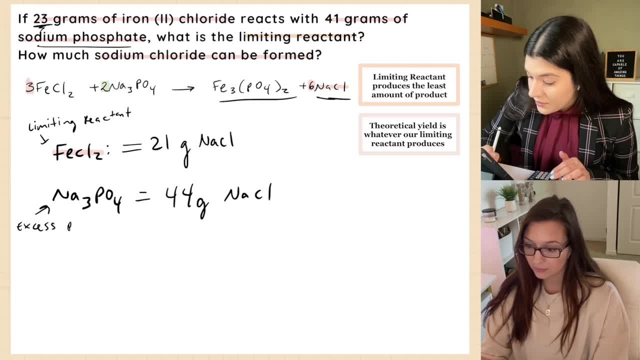 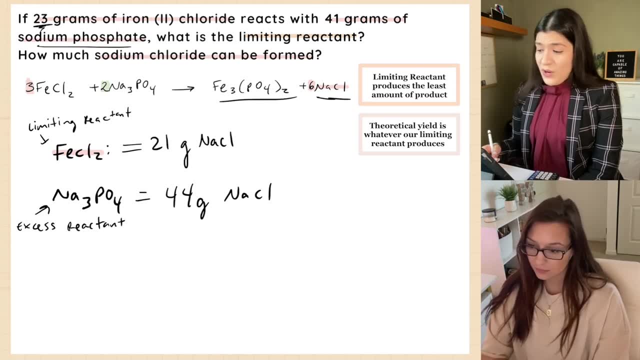 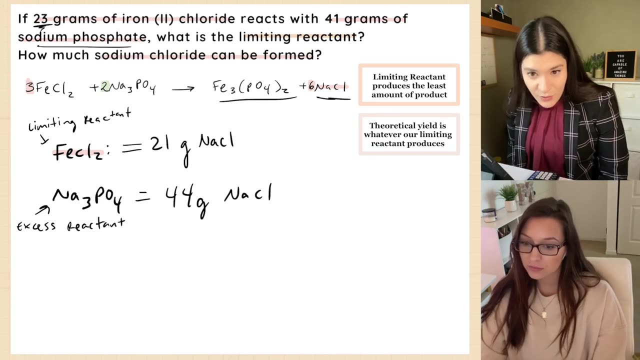 And then this must have been the excess reactant, because it's what's left over Now. the next thing is this is saying how much sodium chloride can be formed. So the theoretical yield is whatever our limiting reactant produces. So what do you think is our theoretical yield? 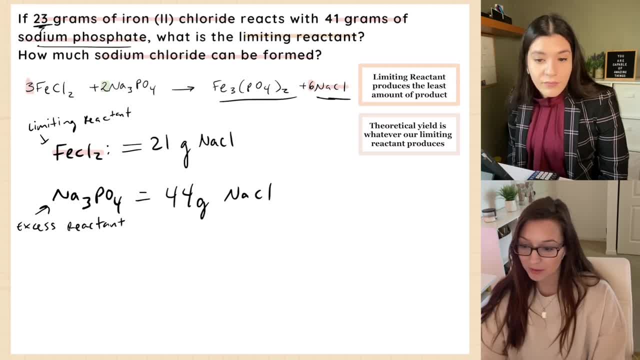 I'm thinking maybe we add them, but I don't know, So we wouldn't add them. So we wouldn't add them. Okay, So what did the limiting reactant produce? Like how much product did the actual limiting reactant produce after we found the 21 grams? 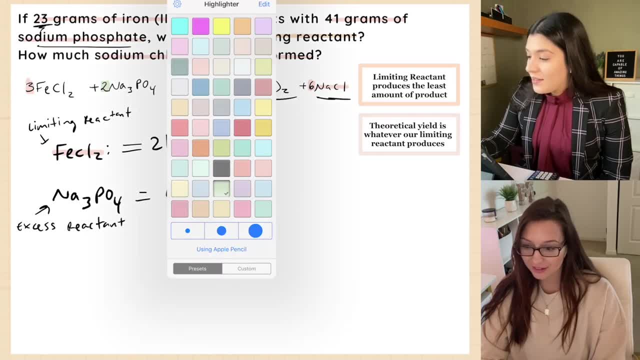 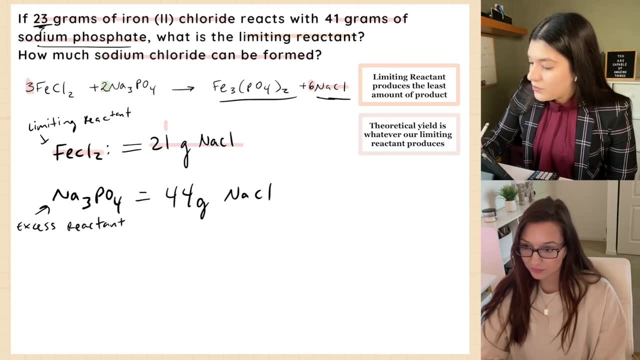 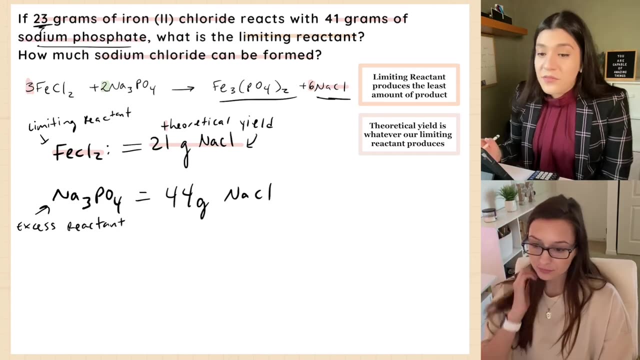 Is that what you're talking about Exactly, Not a trick question. Yeah, Okay, Yeah, So so I know that my 21 grams is the theoretical, is the theoretical yield. So theoretical yield, Now, what is this? 44?? 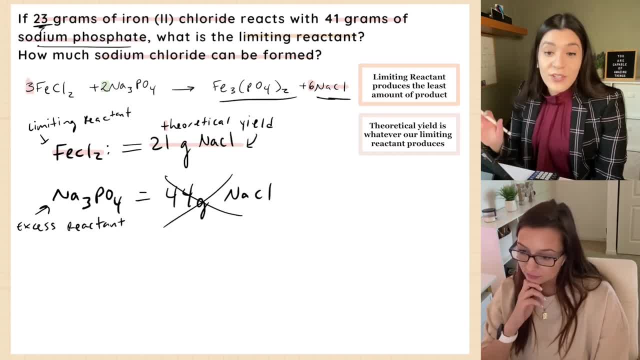 It's nothing It is. it's already served its purpose. The whole point of that 44 was just to figure out what the limiting reactant was. So we do nothing with that 44, erase it from your mind. That is not what we can actually produce. 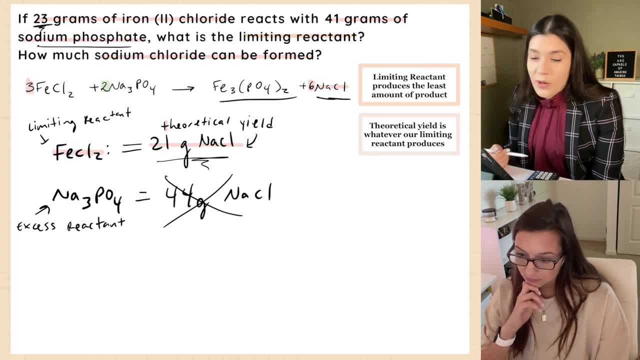 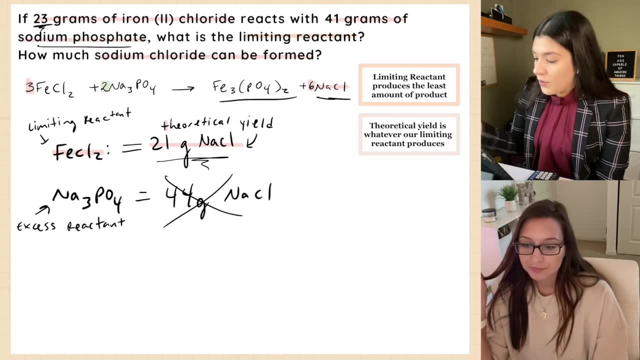 What we can actually produce is the 21 grams of NaCl. Okay, Okay, So that's what answers this question, And then I'm going to keep going. It is going to be important to know what your theoretical yield is. how to find it. 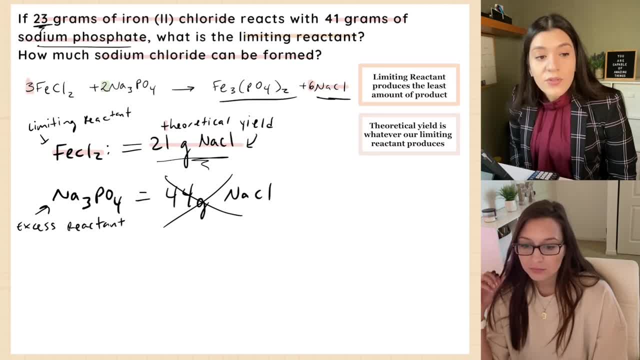 And just like. I'd even say like some of the common words that they use, So they may say like, like in this case, they said how much sodium chloride can be formed. They could have said: what's the maximum amount of product that you can you can form. 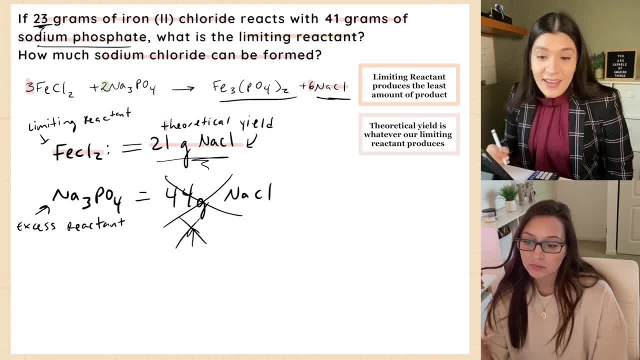 And it's not going to be the largest number. That's not the case. It's always going to be whatever the limiting reactant actually produces, All right. So for every single time they're asking you that they're really referring to the theoretical. 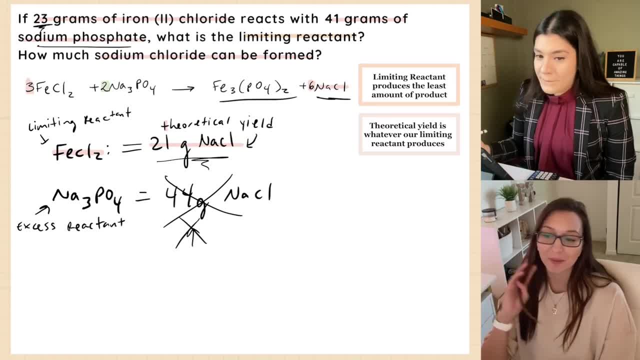 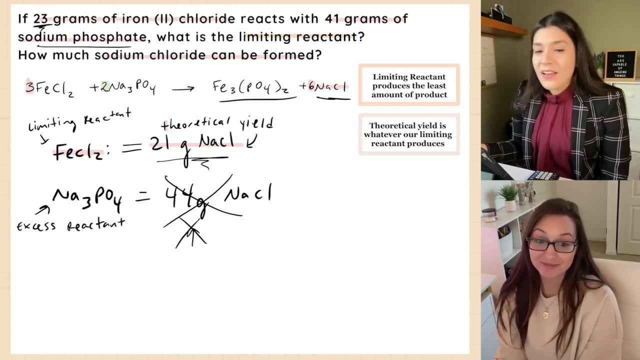 yields. Does that make sense? Yes, I think it meant the bigger number, Right, Right. And even if, like, like it's, they'll say it as like maximum minimum, like all these different things to try to trick you. 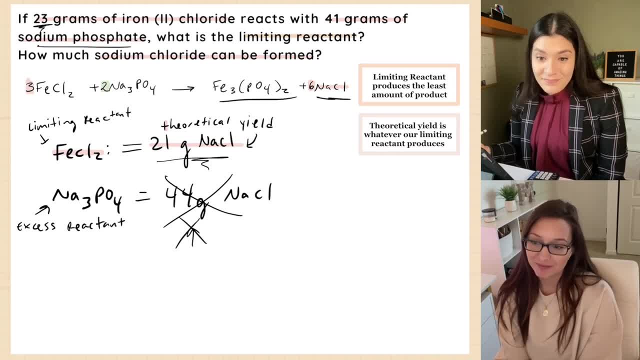 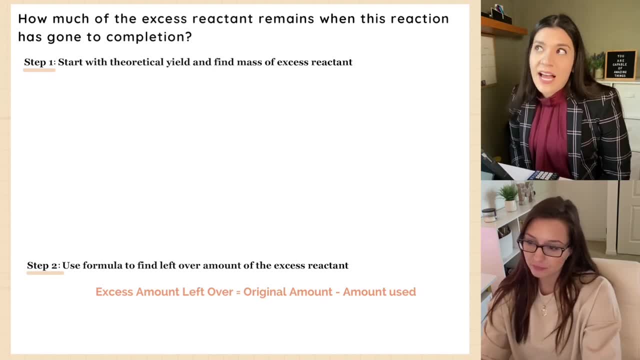 They're all talking about the theoretical yield. Okay, Yeah, Yeah. So the next thing is um talking about the excess reactant and how much is actually left over. So this, this is said this way of saying how much of the excess reactant remains when this: 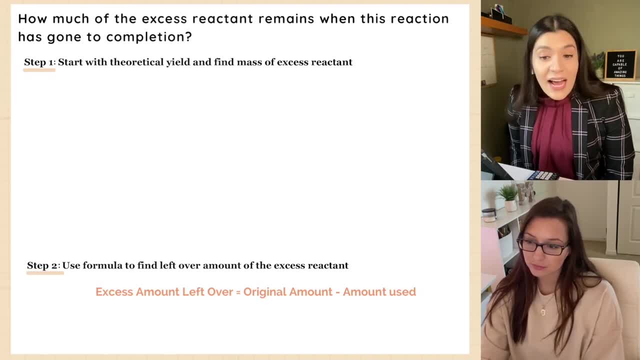 reaction has gone to completion. In other words, how much of our excess reactant Do we have left? And how we do this is we're going to use our theoretical yield. So we take our theoretical yield, which was 21 grams of NACO. 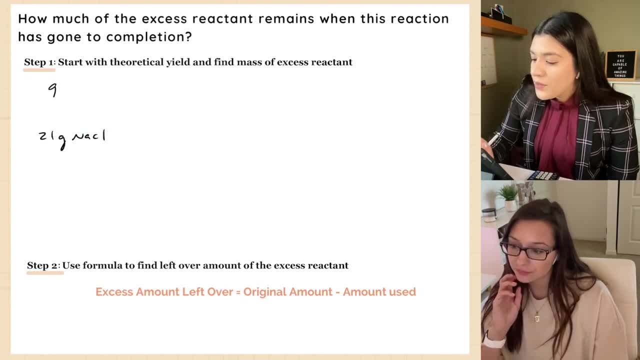 And now we're going to basically go from the grams of our product to the grams of our excess reactant. Okay, So that's how I want you to think of this. This is our product, that we found specifically the theoretical yield, And then now we're going to make our way to the grams. 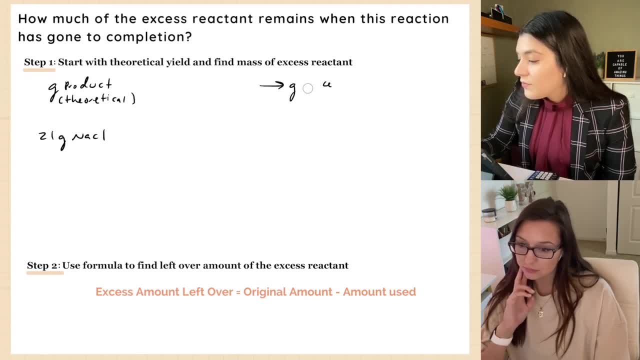 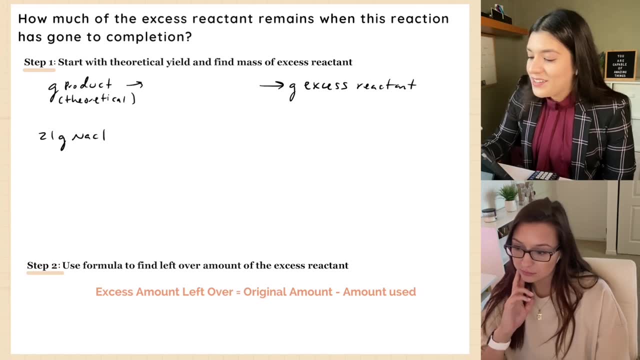 The grams of the excess, whatever the excess reactant was. So I'm going to do this again. It's pretty much almost the same sort of concept, right? We're going to go to moles of our product. It's now like reversed, but we don't have to do this twice. 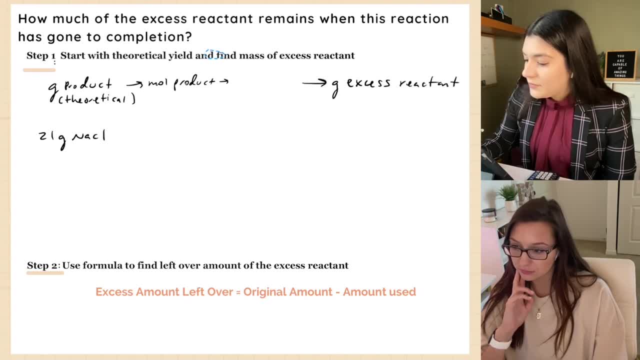 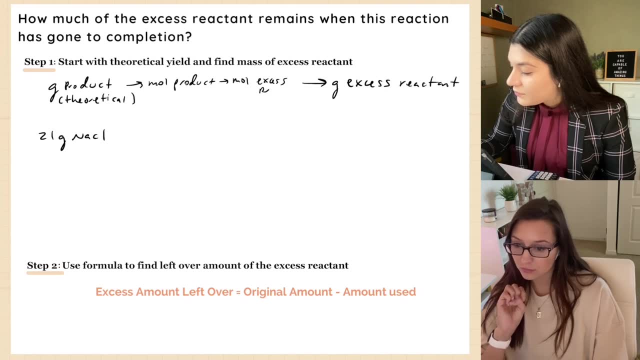 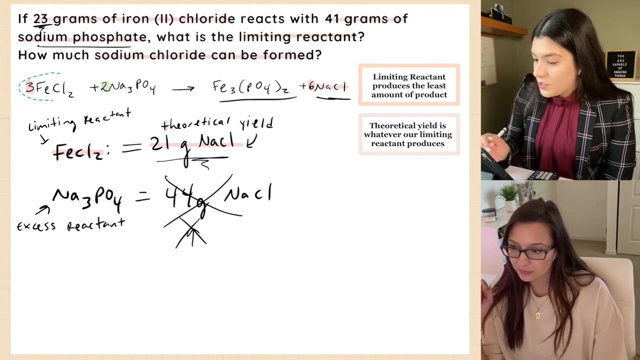 Thankfully this guy wants to slide over, Okay. And then this is the moles of our excess again, excess reactant. Okay, All right. So I'm still going to bring- let me bring back that balanced equation because we will use it again. 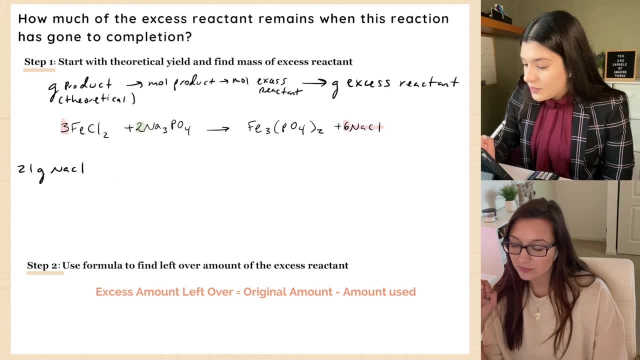 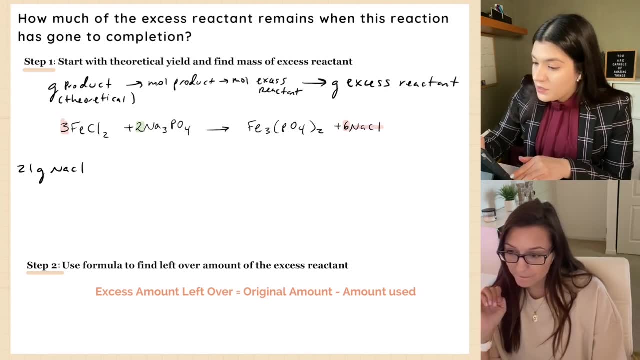 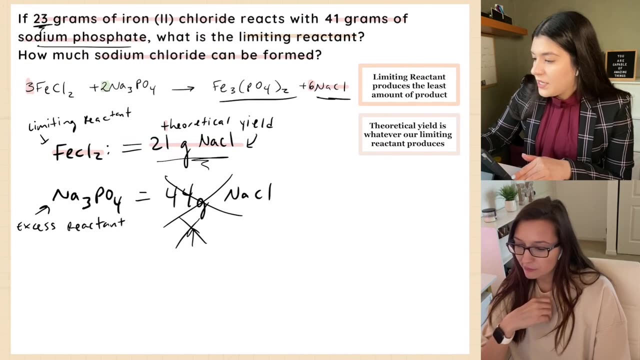 Cool, And same sort of concept. I'm now going to go to the moles of the product, using the molar mass that we previously found. So let me set this up. So I put the grams of NACL and I'm just going to take it from what we found. 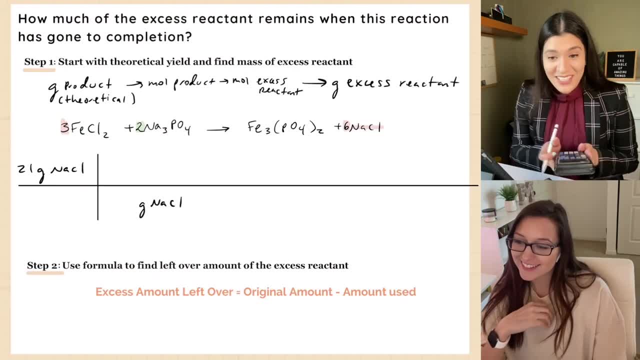 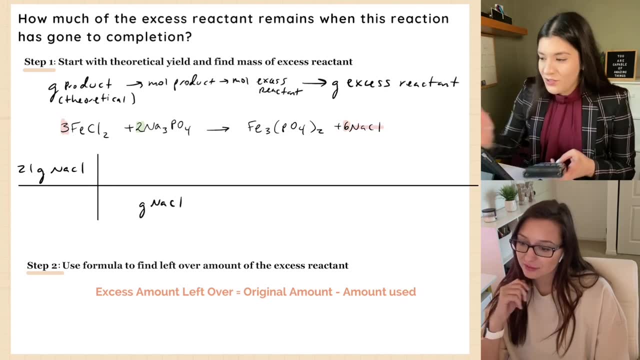 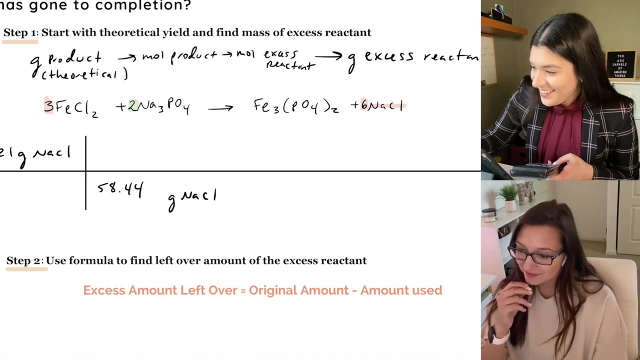 Actually, I deleted it. I deleted it, Nevermind. Okay, I have to redo it. So that was 22.99 plus 35.45.. I used to have a lot of these memorized back when I was like tutoring, every single day. 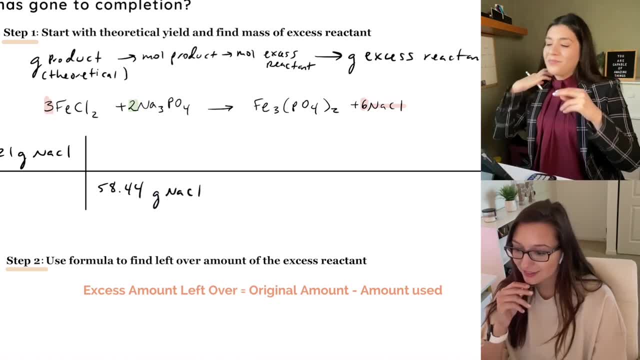 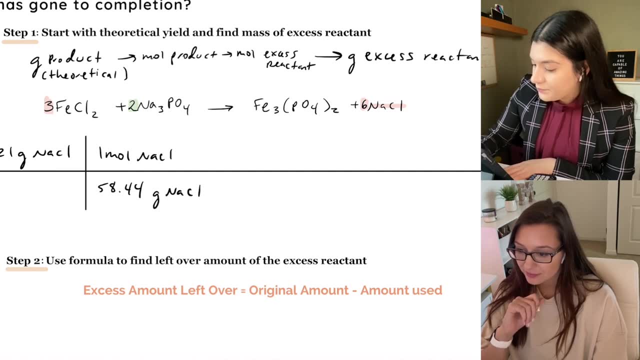 It's like coming back to me again. Okay, So cool. That was 58.44.. And this is for one mole of NACL- Awesome Now. So the next thing is going to the moles of our excess reactant. 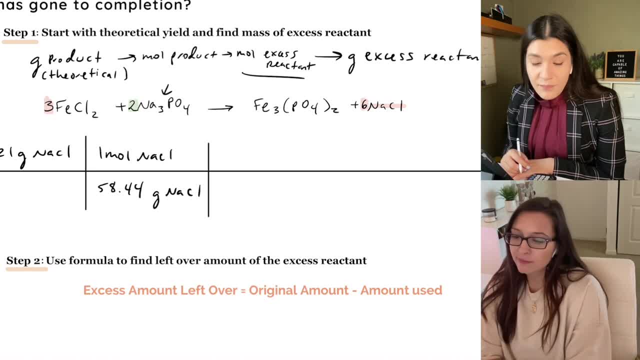 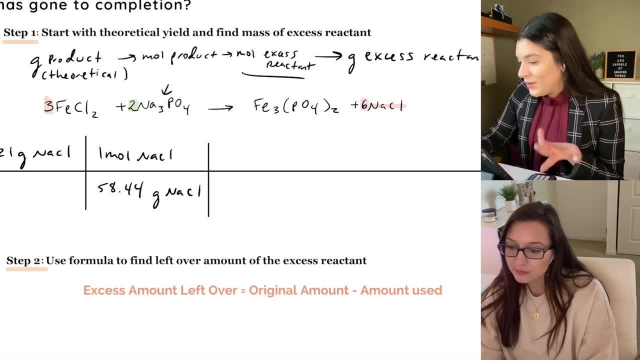 So we said that our excess reactant was this: one was sodium phosphate. So I need to go to the moles of sodium phosphate. I'm going to look again at the periodic, I'm going to look again at the balanced equation and say that this is six moles of NACL. 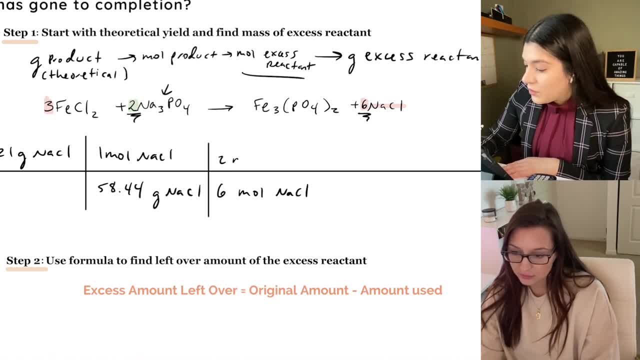 And then now I'm trying to get to the excess reactant, So two moles of sodium phosphate, And last I would use the molar mass of the excess reactant to give me the grams. So I'm going to do this again. 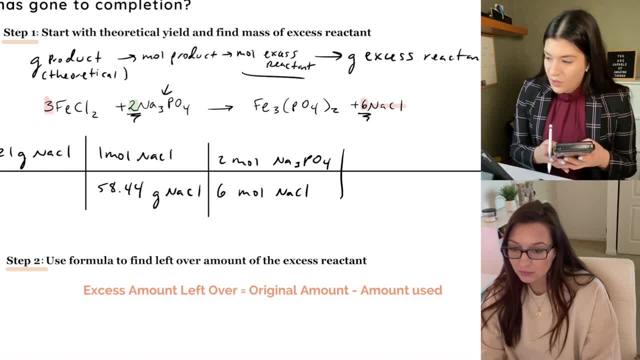 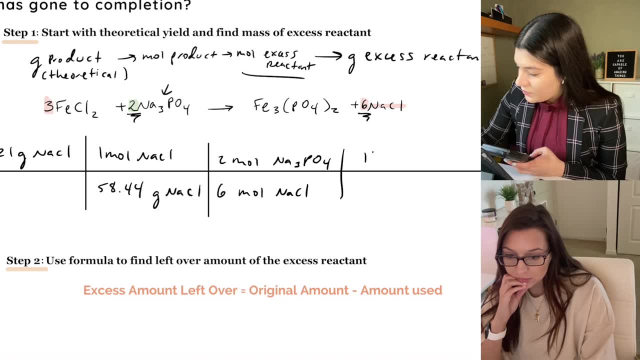 Just finding this again. This was what 22.99 times three plus plus, which was 30.97 plus four times 16.. So it was this 163.94 grams of this. Okay, A lot of stoichiometry, Yeah. 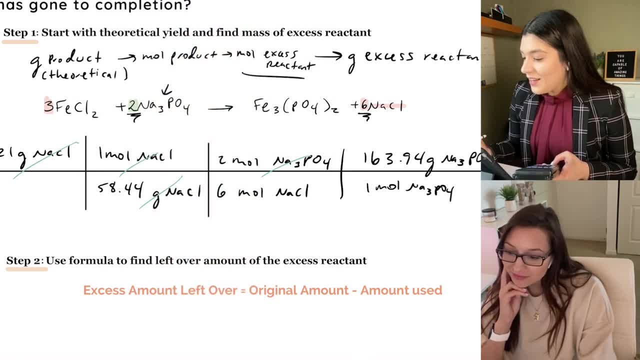 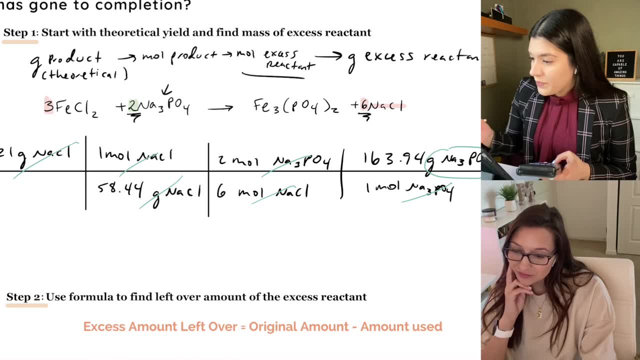 So I'm going to cancel everything out And I'd see that, Yes, I have what I'm looking for, which is the grams of my excess reactant. The next step is to just multiply. So I'm going to multiply everything out. 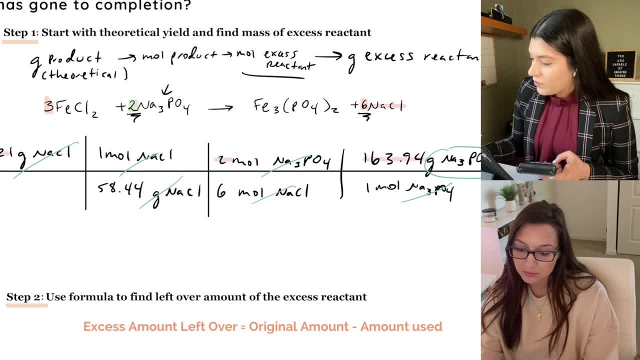 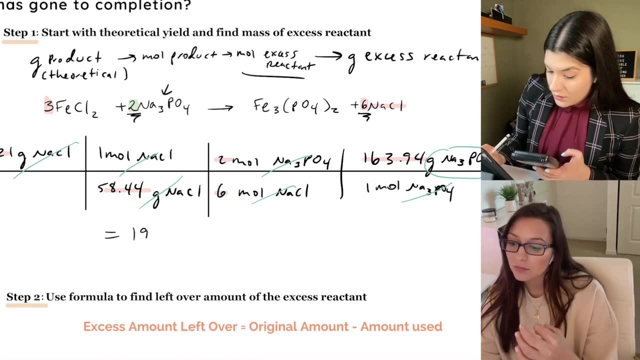 Doing this top front first, 21 times, two times all of this Divided by the bottom multiplied, So these two multiplied And I would get 19.63.. I'm going to round to two sig figs, since this starts off as two sig figs. 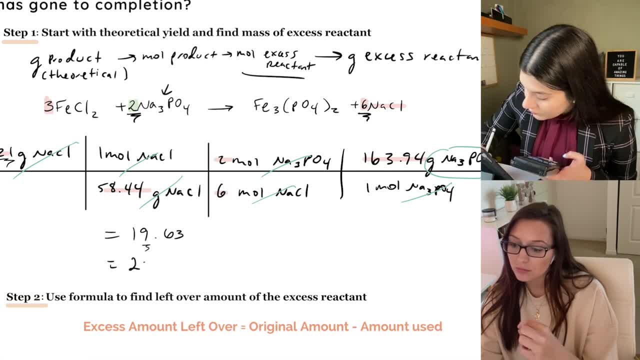 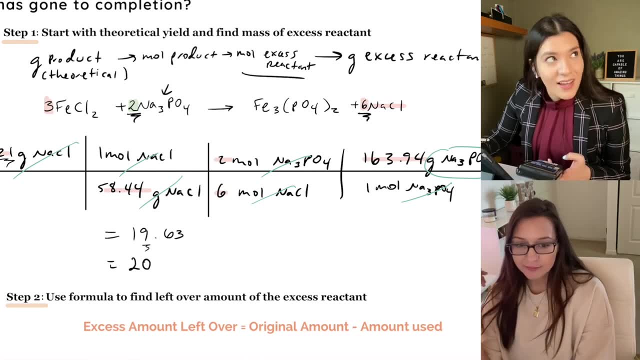 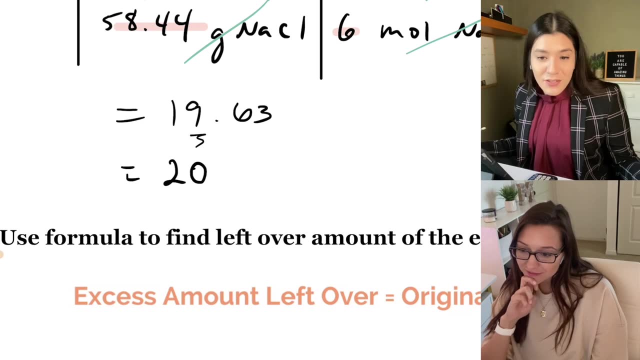 So I'll round up to 20.. Which technically isn't Two sig figs. Yeah, But I still would round up. So I would still round up regardless. I'm not going to change this to scientific notation notation, Which is what you would essentially do. 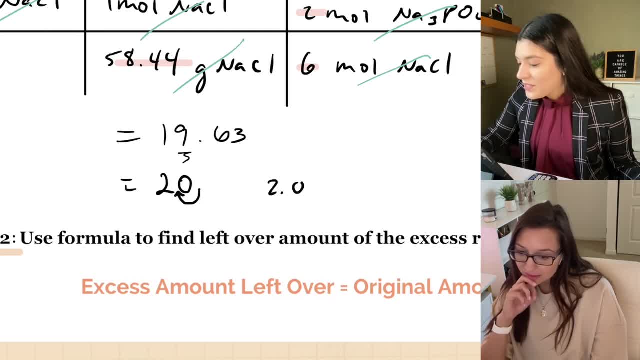 You'd move this over once, Like if you're really being a stickler, but that's not what we're looking for right now, And you'd move this, You move this over once. So negative, Actually a positive one, If, if it was truly scientific notation and you needed to end with that answer: but we're 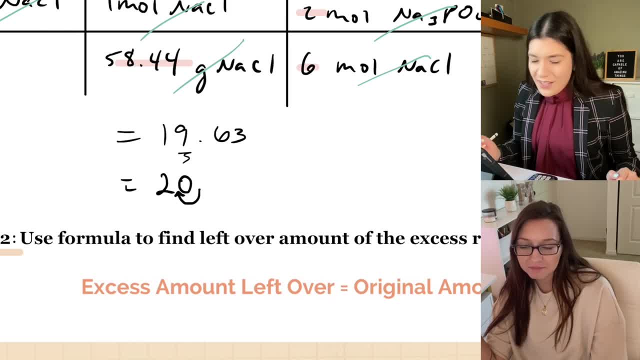 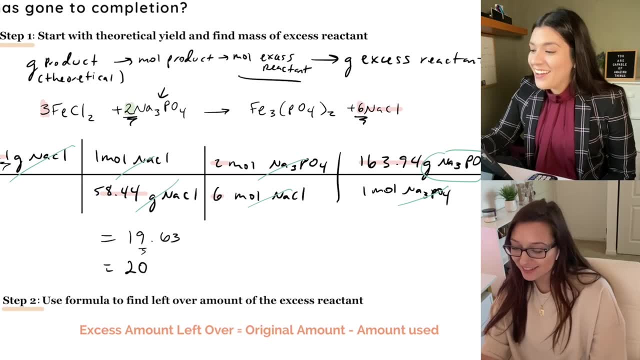 not ending with that answer. Answer: Okay, Does that make sense? Yeah, I'm just going to say 20.. For everybody who wants to be a stickler with sig figs and call me out, So I, if you really want it, you'd put 2.0 times 10 to the first. 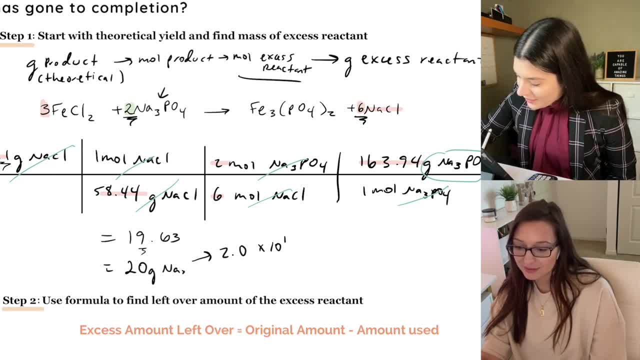 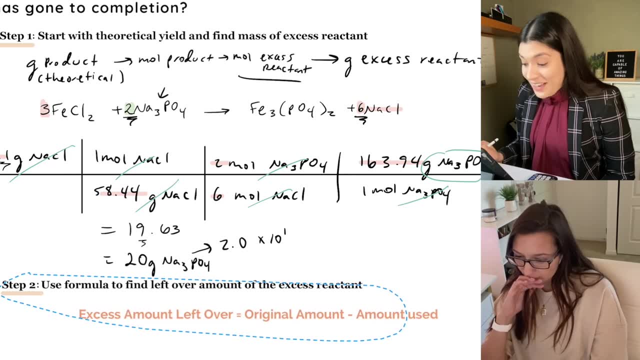 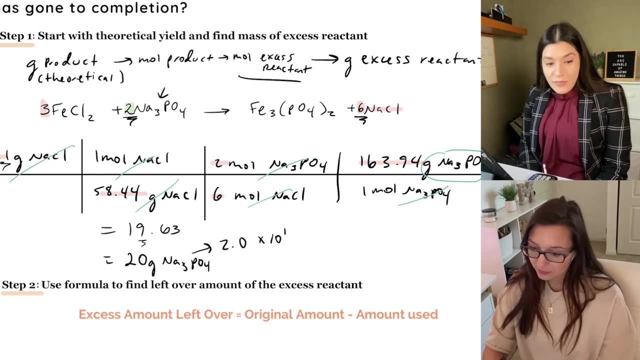 Okay, And this is grams of NA, three, PO four, All right. Next step- Finally- we're almost done- is to actually find the leftover amount of the excess reactant. So what we do now, what we just found, what was actually used in the reaction, 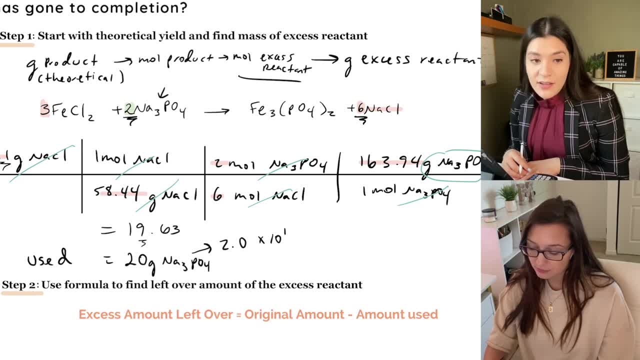 Okay, So think back to the like, the lattes, and we had two cups of milk And we had our brood coffee. So it was actually used was two cups of brood coffee to make two lattes. Correct, This is what we're saying here. 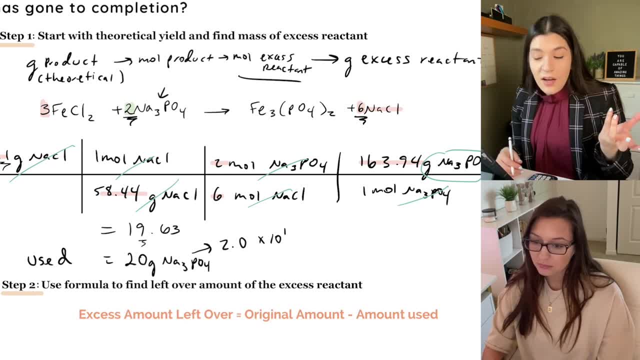 This is the amount of the used amount of our excess excess reactant. So now we're trying to figure out how much is left over, So I'm going to take the original amount that they gave me in the question, which was a 41.. 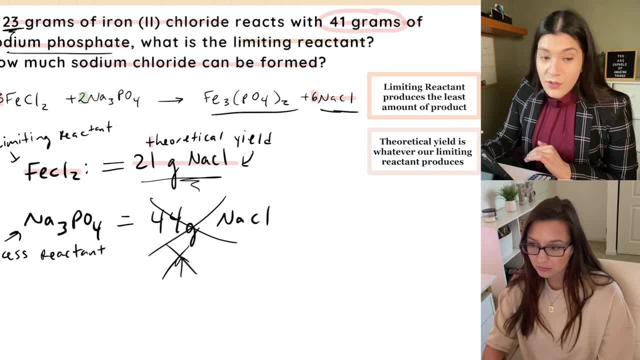 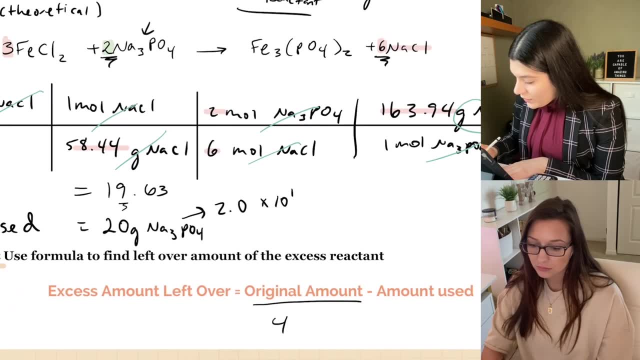 So I'm looking at this. So, 41 grams of sodium phosphate- That's what I started off with and I'm here. So I'll say, okay, I have 41 grams and I'm subtracting this by what I just found. 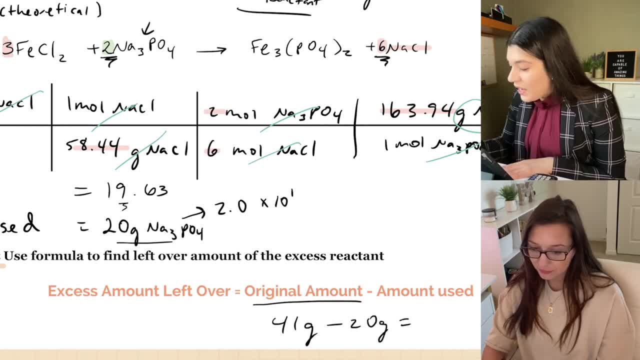 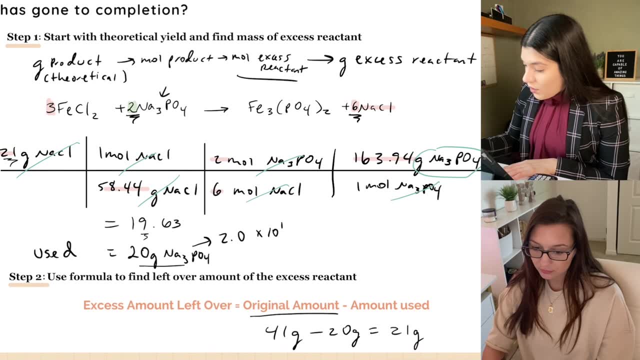 So the amount used, which was 20 grams, And then now subtracting that we don't need a calculator here, right, This is just 21 grams that is left over. So our, our answer here would have been that there's 21 grams of NA three PO four. 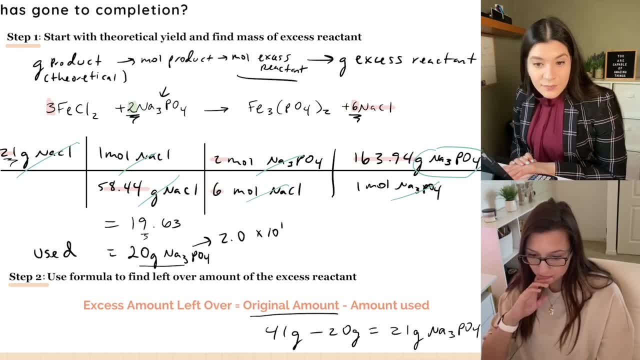 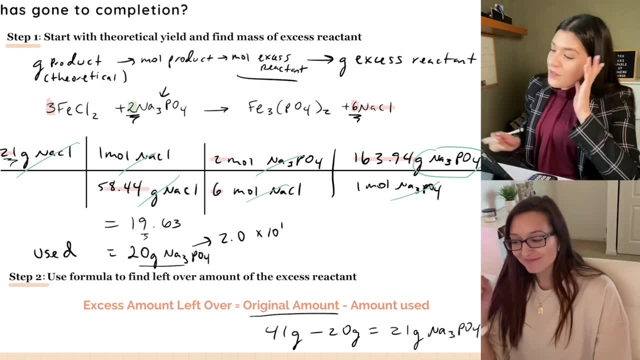 And that's, that's how much is left over. Okay, Makes sense. Yeah, This isn't like, really it's a lot of stuff, but I know, I, I trust me, I know I know this is this is why we're covering it and going, you know, going over. 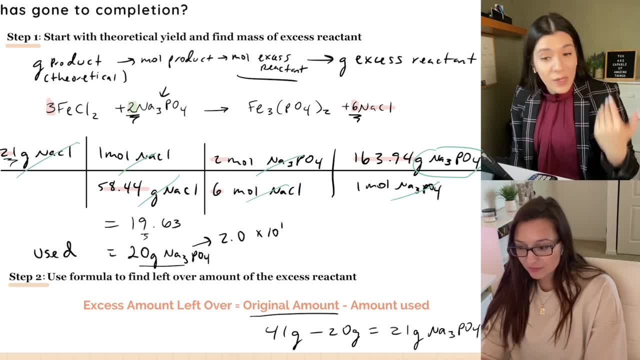 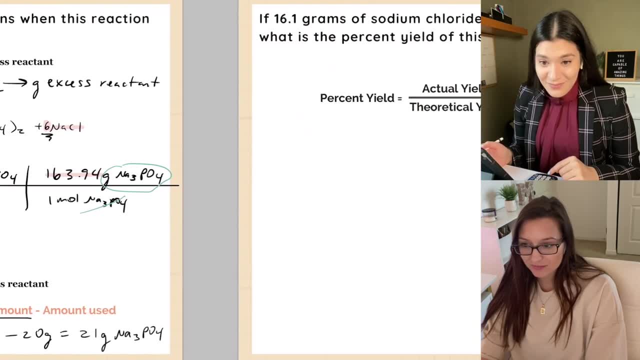 every single thing you may see. So I put out the steps. this is going to take practice, as everything does, Um, but we're we have one more type of question that they could ask with this section. Okay, Okay, So I'm going to keep going. 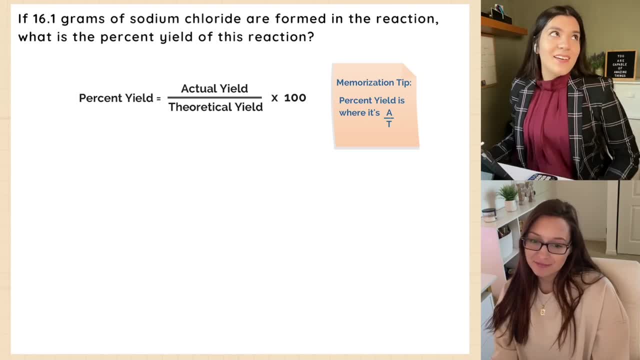 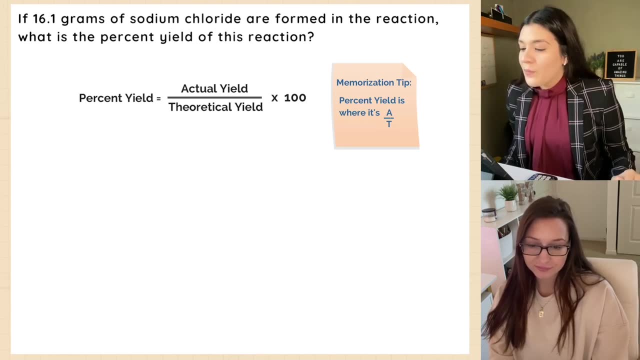 I know this is like these questions tend to be like, uh, multiple, Like when they have like multiple parts like a through, like D. So yeah, that's something to be aware. Um, this question is saying if 16.1 grams of sodium chloride are formed in the reaction. 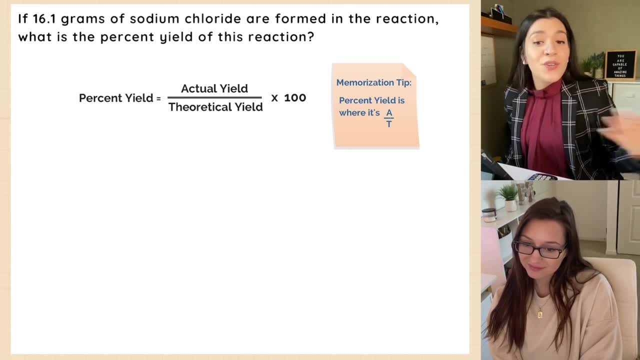 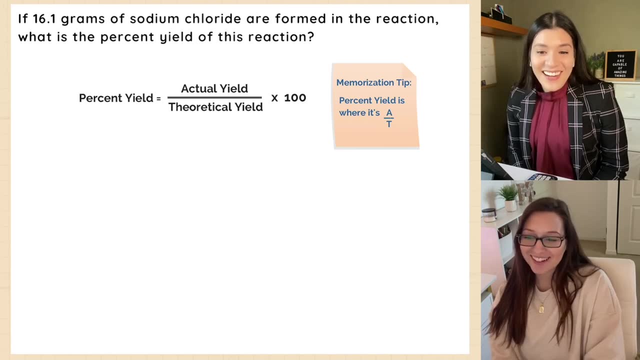 what is the percent yield of this reaction? So you've done percent yields, most likely in lab, already. uh, that smile tells me: yes, So I'm talking, I'm laughing at. percent yield is where it's at. Oh my gosh. 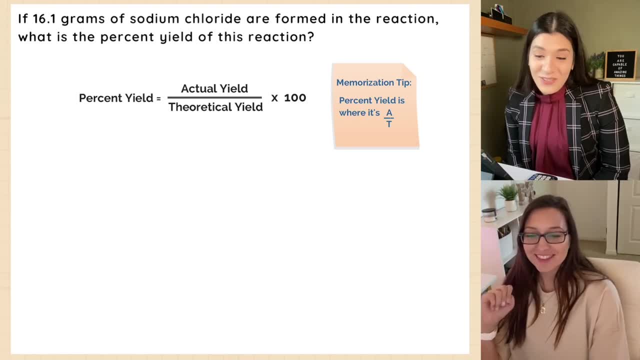 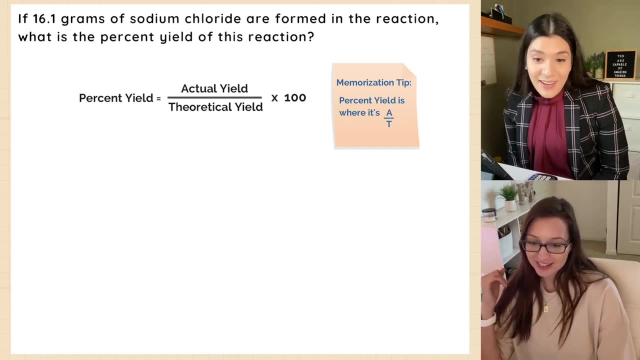 Okay, I'm glad, I'm glad, I'm like this is going to be nerdy or door, I don't know. Dorky, That's amazing. I'm going to remember that. Okay, cool, Awesome. So that's how I remembered it. 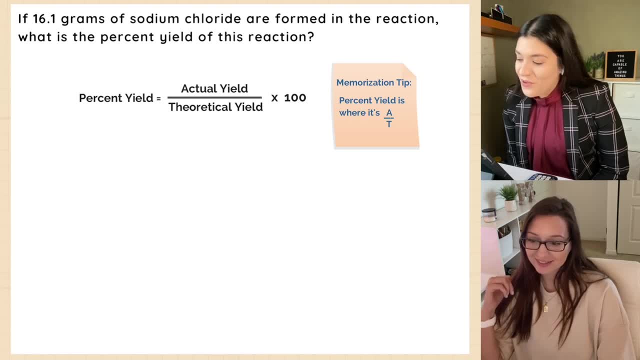 Um, I laughed when I thought of it and yeah, so yeah, that that's the trick for for what this is, It's to remember the formula Um, so you never forget the formula. percent yield is where it's at. 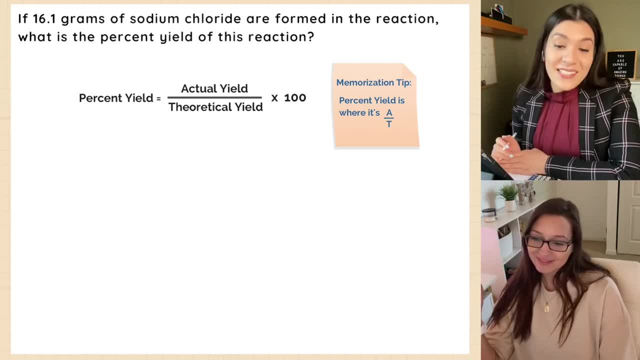 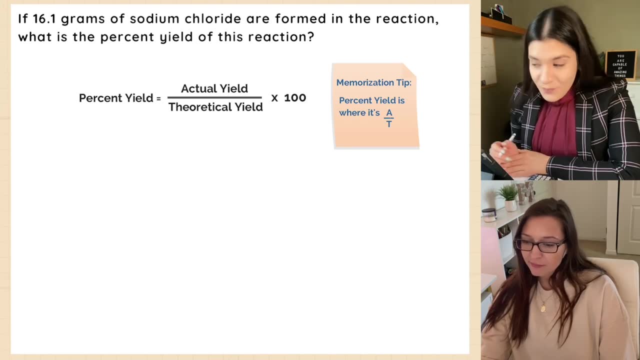 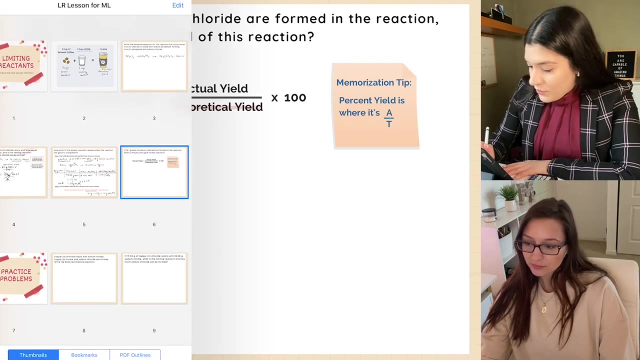 Cool, Um. so besides the formula, you have to understand How do I identify what the actual yield is and what the theoretical yield is. So we already found in this question what the theoretical yield is right. So, going back to what we found, we found that 21 grams of NaCl was actually was produced.